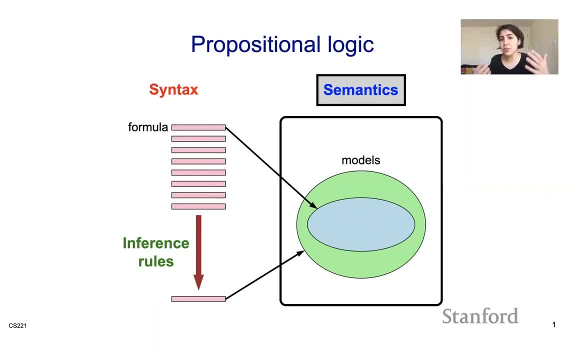 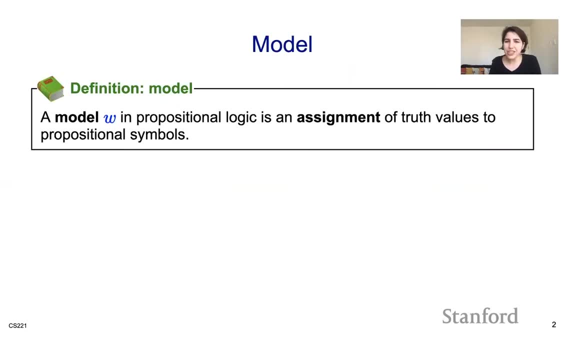 syntactical formulas that we defined And that corresponds to semantics. So in this module we are going to be talking about semantics and giving meanings to those formulas And, in general, in this lecture we are going to have a good number of definitions. So I'm going to write. 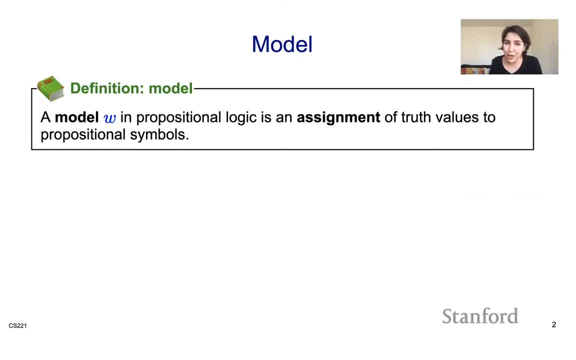 out those definitions in a separate whiteboard so we can keep track of them. But a good number of definitions are coming, Especially in this module, And let's start with some of them. So the first definition is a definition of a model, And this is a very poor choice of words. We've been using the word model. 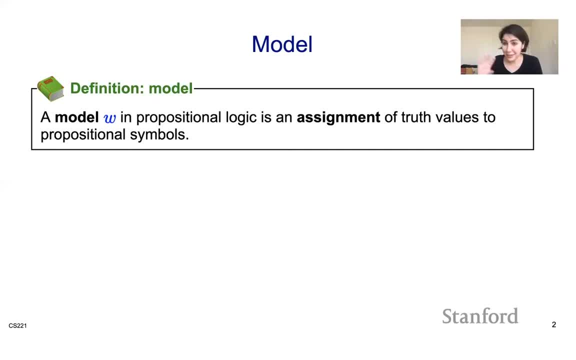 throughout the lectures of this class as a different thing. right, Like, we talked about modeling, inference and learning, But in the logic lecture we're going to assign a different meaning to the word model, And that has historical reasons because historically, like model has been. 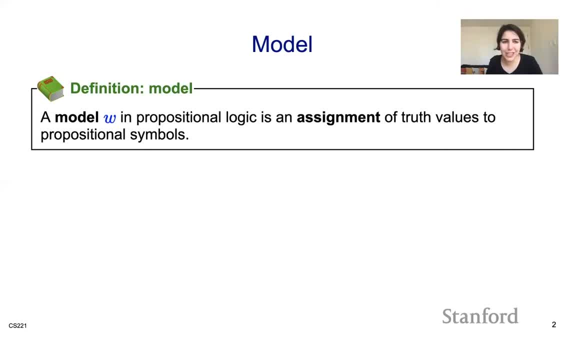 used in these settings For in logic, in this particular way to refer to assignments really. So a model for this lecture and for the logic lecture, let's refer to a model in propositional logic as an assignment of truth values to propositional symbols. So I'm going to use the word W for a model, W for world. So that's. 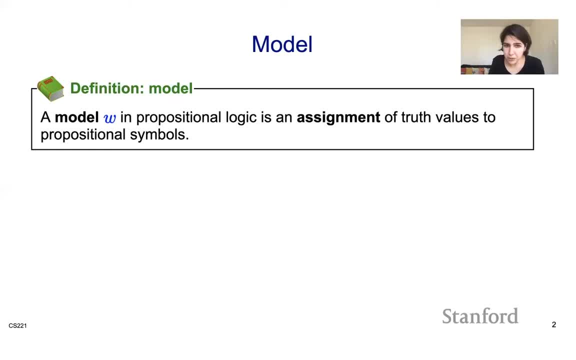 why it's called W. So a model W in propositional logic is just an assignment of truth values. Okay, so what does that mean? So let's look at an example. For example, let's say we have three propositional symbols: A, B and C. 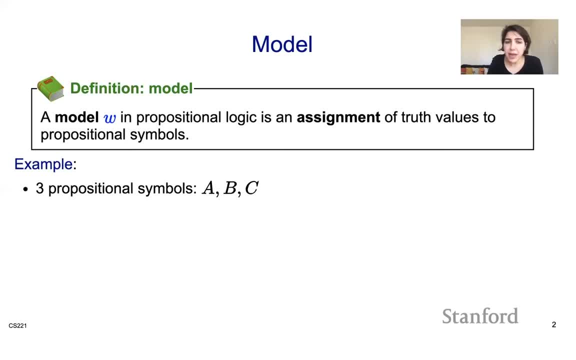 Okay, how many models do we have? Well, we can have eight possible models, right Two to the three possible models or worlds that we can live in, And a particular W, a particular model is going to be a particular assignment. So, for example, I can pick A equal to zero, B equal to one and C equal to. 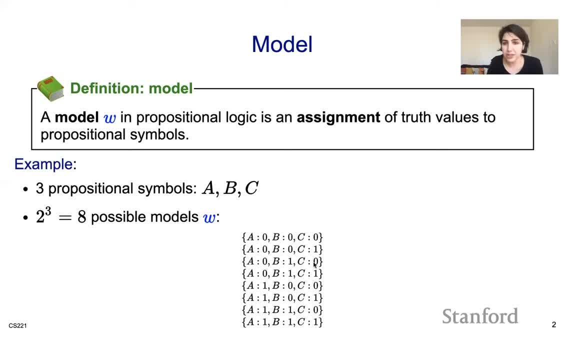 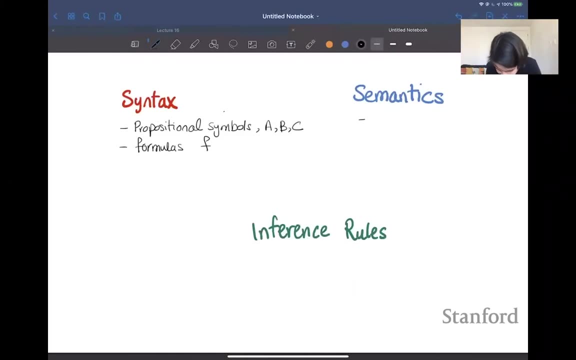 zero And that's a model. That is one W that corresponds to an assignment of truth values to propositional symbols. Okay, so let me write that on our whiteboard here. So, going back here, I'm going to start under semantics And then we have the word model, Model, And I'm going to use the word W for it. 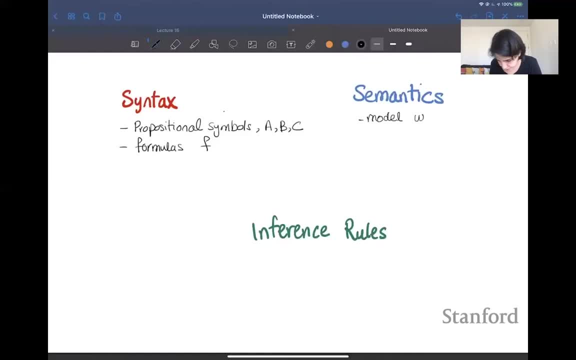 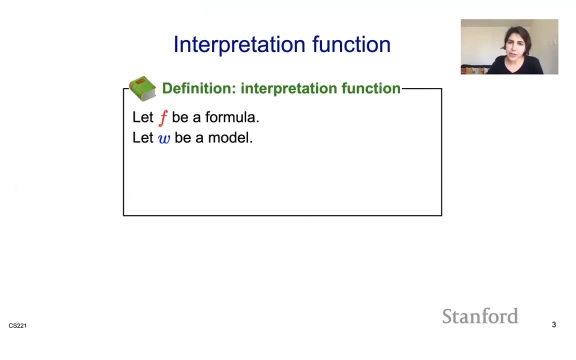 Okay, All right, Let's go back. All right. So now we are ready to define this thing that's called interpretation function, And an interpretation function is the thing that actually gives us semantics and gives us meaning. So what is an interpretation function? So, let F be a formula. That's what we defined in. 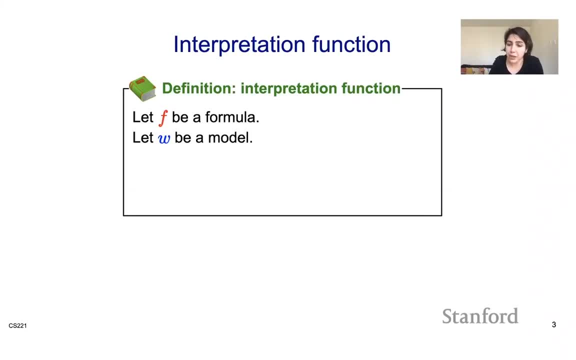 syntax And let W be a model. Okay, So an assignment, So an interpretation function. I gets a formula, gets a model, and it basically outputs true or false. It basically tells us if, if W satisfies F or if W doesn't satisfy F. Okay, So so interpretation function. 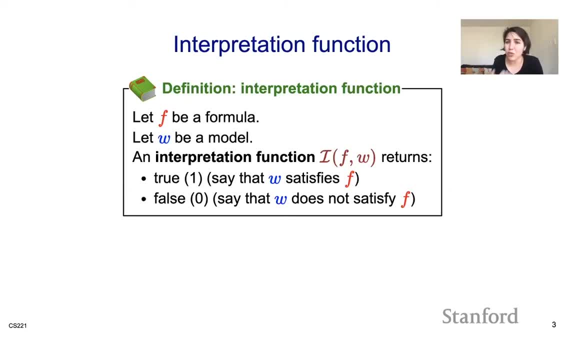 is really the thing that binds formulas and models: Formulas living in the syntactic syntactic land and models living in the semantic land, And and basically interpretation function is trying to, like, connect them and tell us if if that is true or not. So 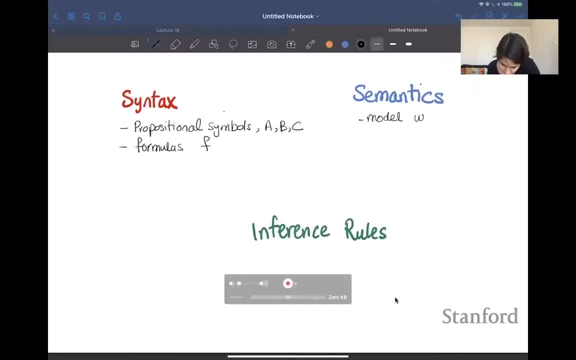 so let me go back here and let me let me write out interpretation function. So it's a function I that takes F, the formula, and W and it gives us true or false. So let me go here and show this. So let's say that we have a formula F, I'm going to write or draw our 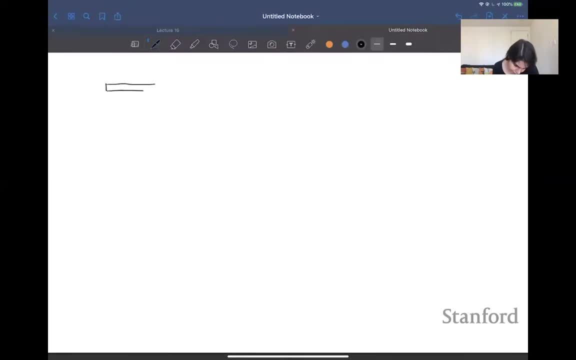 formulas using these rectangle rectangles. So in the, in the syntactic land, you might have a number of formulas. Let's say, I have one formula F and I have one formula F, So I'm gonna write out a formula and write out what the formula is. So this is a formula. So this is a formula to keep. 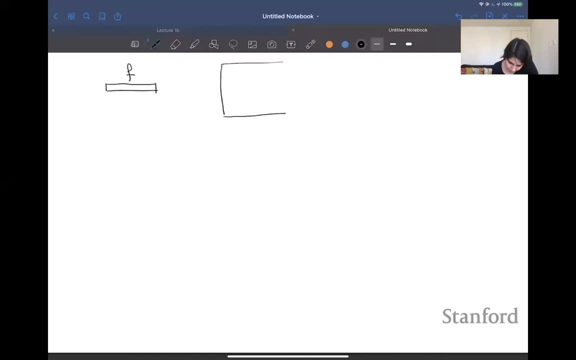 And then the world of semantics. we might have different models, right, These are different models, or worlds that we can live in, or worlds, And I can pick a specific one. Let me call that W. Okay, let me call that W. 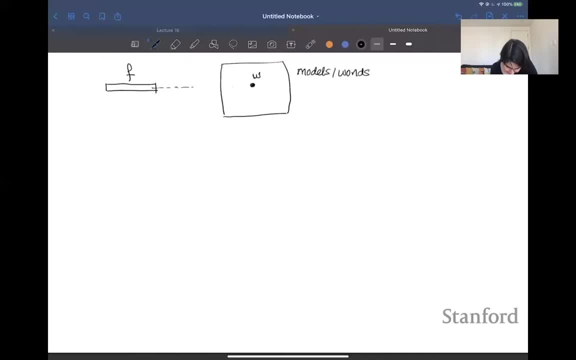 And what I can do is I can basically connect a formula to this W using this interpretation function. So I'm gonna have an interpretation function- F and W- that gives me true or false, if F satisfies W or not. Okay, I can have other Ws in this space of models. 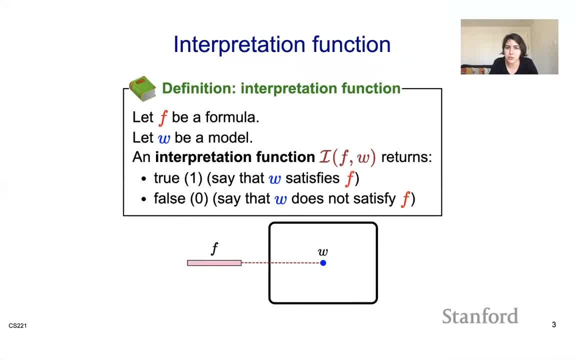 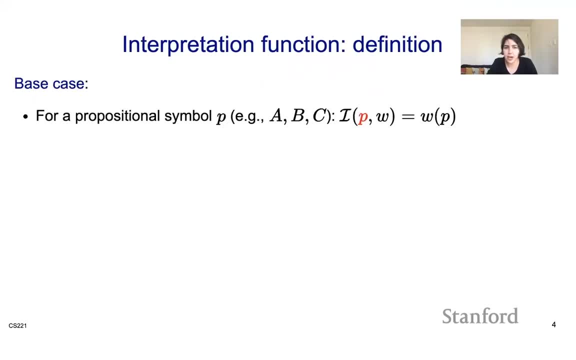 in this semantic land. So how do we define an interpretation function? So the way we define an interpretation function is recursively, in a similar way that we defined our syntax. So we're gonna start with propositional symbols. So we have these propositional symbols. 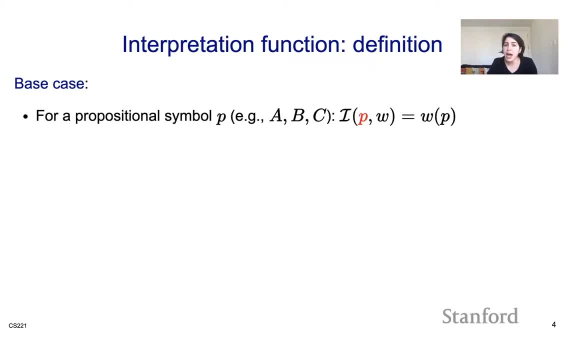 A, B and C, Like these. take Boolean values and the interpretation function of each one of these. each one of these propositional symbols, P and a model W is just going to return W of that propositional symbol. Okay, remember, W is an assignment to these. 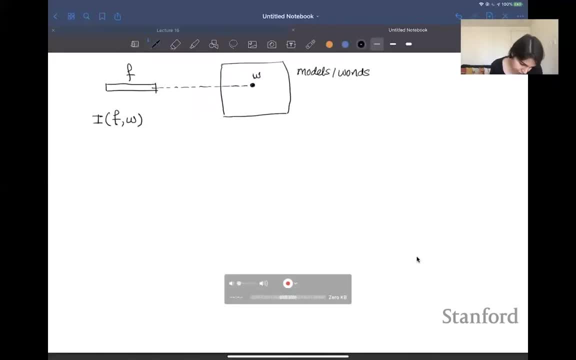 So, going back here, let me give you an example. So my W is going to be an assignment that maybe says A takes the value zero, Okay, and my propositional symbol is just A right. So if I look at interpretation function over P and W, 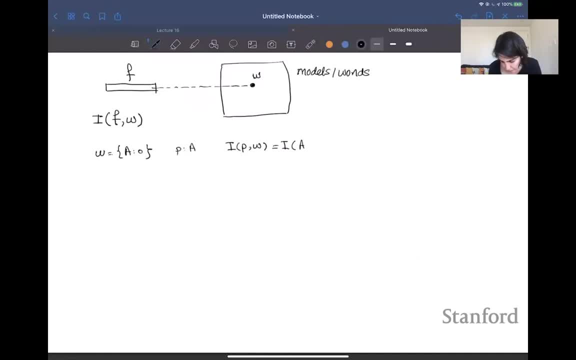 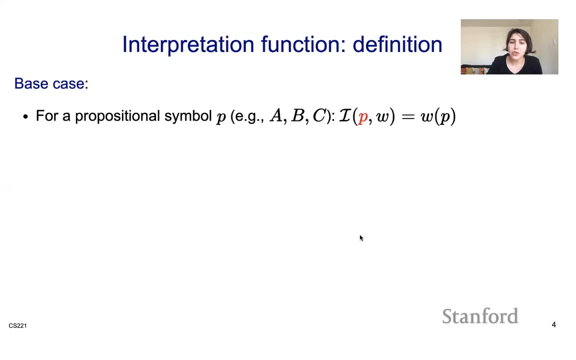 it's basically checking interpreting A and the model A being assigned to equal to zero, and that returns the value zero. Okay, so that is just for the base case of this. okay, So then, when we think about more general formulas, these formulas, how are they defined? 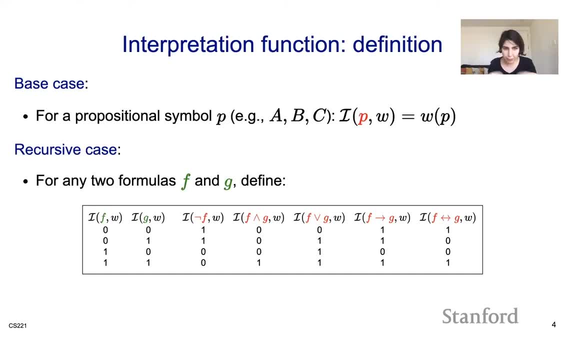 They're defined based on these logical- you know, logical- connectives used applied over propositional symbols, And based on that we can basically recursively define this interpretation function. So I can have a formula F and a formula G and I can create kind of this truth table. 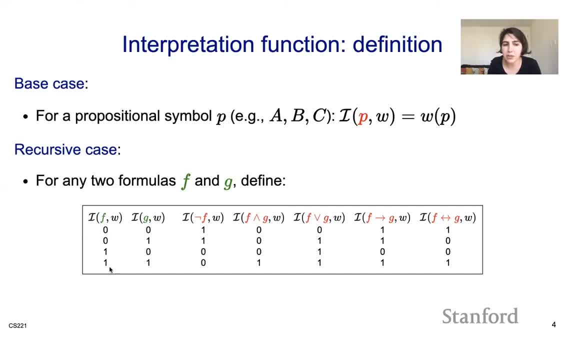 and interpretation function of F and W could take values zero or one interpretation function of G and W could take values zero, one, And then for anything else, like for any of these other logical connectives, I can basically recursively define them. So what would be an interpretation function? 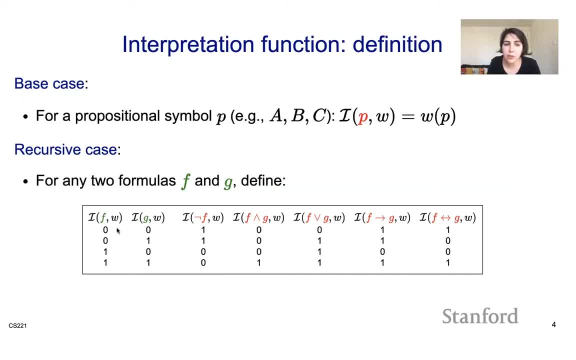 Okay, So what would be an interpretation function, function of negation of f and w? it would basically try to negate this column, right? So it would be 1, 1, 0, 0. Or if I'm thinking about interpretation of f and g, well, what would? 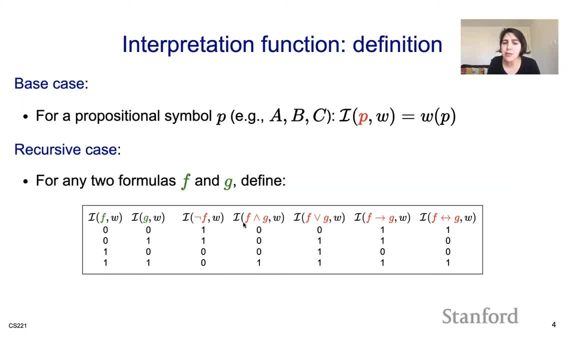 that be. And the model w? what would that be? That would be interpretation function of f and w and interpretation of g and w, So basically adding these two columns and that gives us these values, and so on. Similarly, we can define interpretation function over f or g, or f implying g or f. 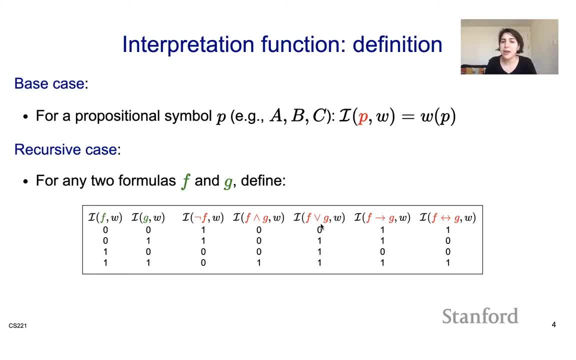 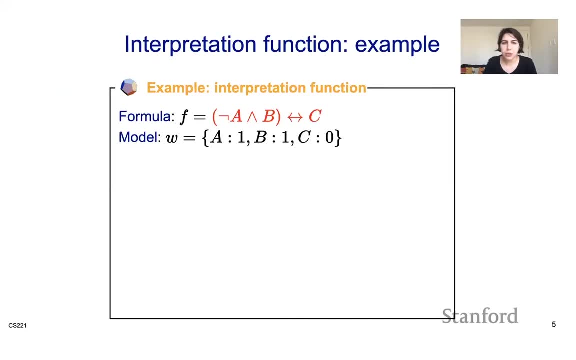 bidirectional implication of g and so on, And then we can kind of assign meanings to these more generic formulas. okay, All right. So let's look at an example of how do we do this recursively. So let's say we have a formula f and that formula is negation of a and b. 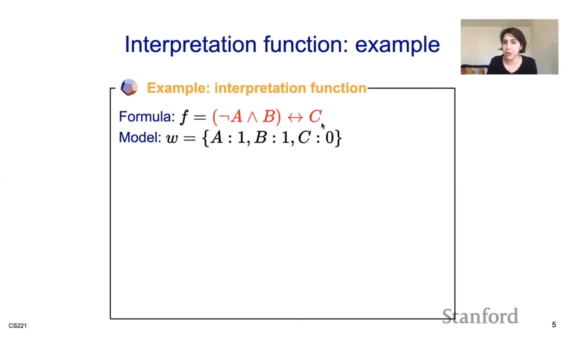 and bidirectional implication c. okay, So that's my formula. I have an assignment, I have a model. That model is truth, assignment to my propositional symbols a, b and c. So let's say a is 1, b is 1,. 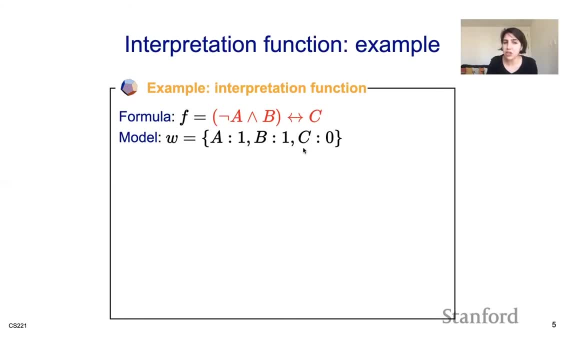 and c is equal to 0.. And now I can call an interpretation function f and w and see what the value of that would be. How do we do that? Well, let's start with these notes. So at this note I can call interpretation function over symbol a and w. What is that? equal to? Well. 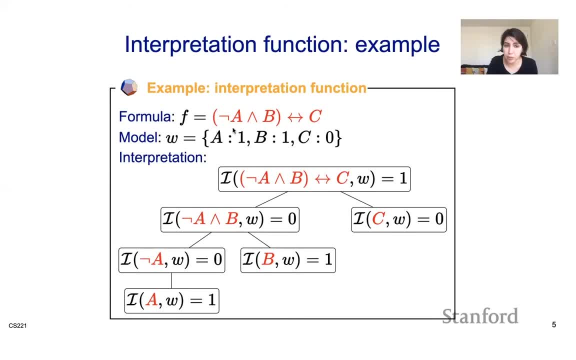 that is equal to just 1, because I'm just going to call my table of models right, I already have this. That's just equal. So that's equal to 1.. Then negation of a is going to be equal to 0.. What is interpretation? 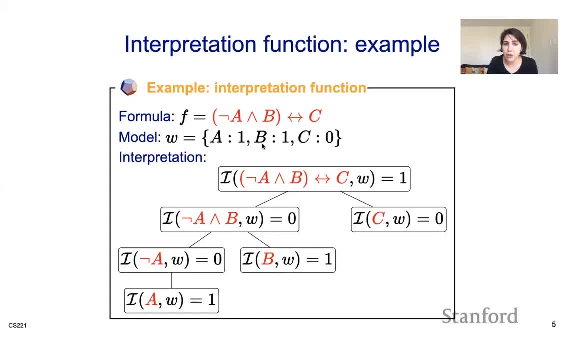 function of b and w. Well, again I have an assignment, I have a model That tells me b takes value 1.. So that's 1.. And then, if I'm taking an interpretation, function of negation of a and b. 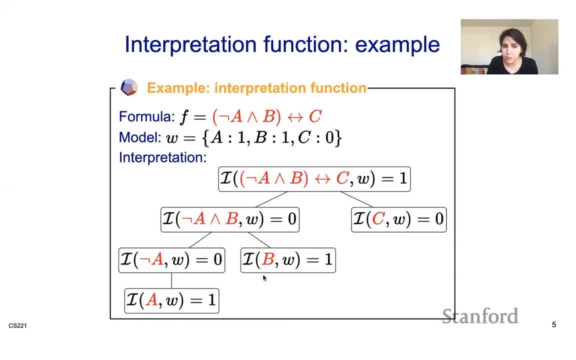 then that is the end of these two. So 1 and 0 gives me 0.. Similarly, I can look at interpretation function of c and w. reading that off my model, That is equal to 0. And then when I'm looking at, 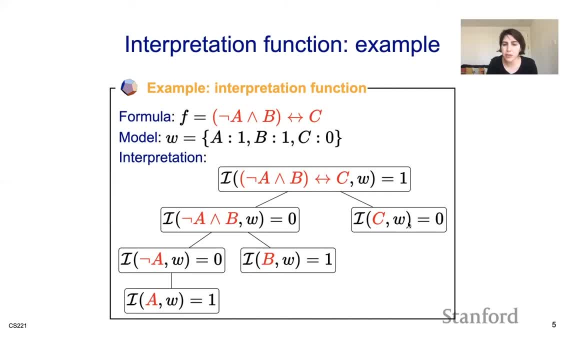 a question. I can call interpretation function of b and w, So that's 1.. And then if I'm taking an interpretation function of c and w, reading that off my model, that is equal to 0. And then negation of a and b. well, these two are equivalent, So that's just going to be equal to 1.. 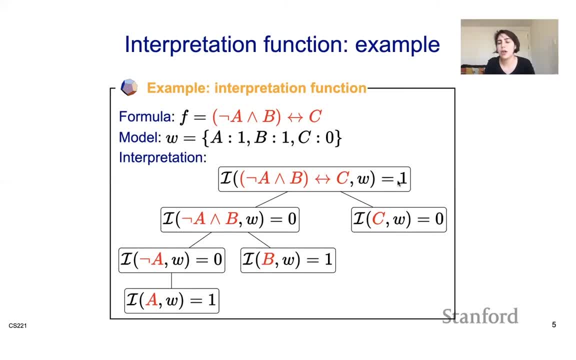 So this is just showing recursively how do we run interpretation function. So there's no learning here. This is defined by logic. You can define your own logic- That would be fun- But this is defined by some sort of logic. that is this propositional logic that you have. 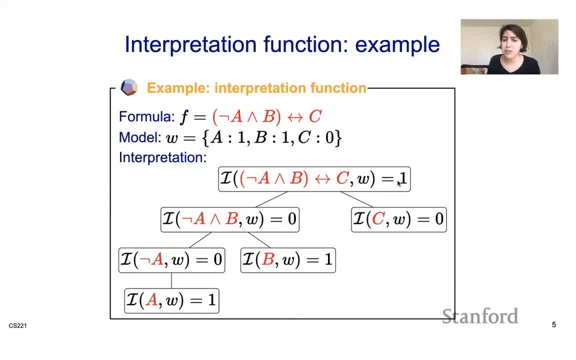 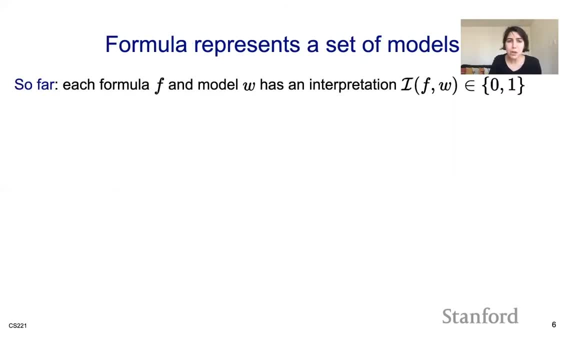 defined using our formulas and using our connectives and so on. And I'm just calling this, I'm just computing this, So I'm not doing anything like fancy here. okay, All right, so each formula and model, right like we'll give, like we can interpret it using this interpretation function and that gives. 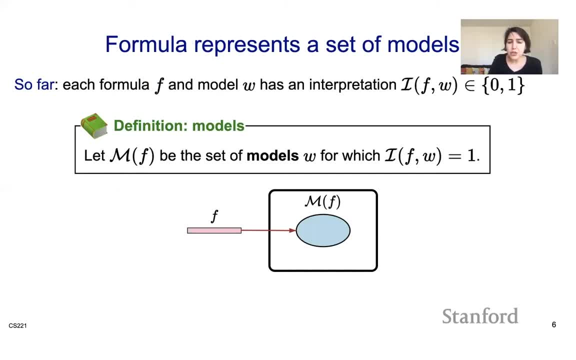 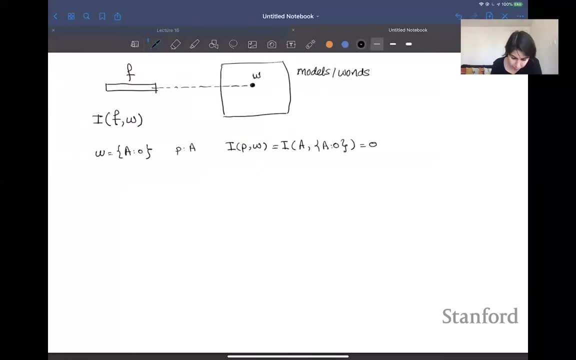 us a value, zero or one, okay. So now I'm going to define this thing that's called models of f and basically it's a set of w's. It's a set of models where interpretation function is equal to one. So, going back here, right like looking at this, there could be one w. 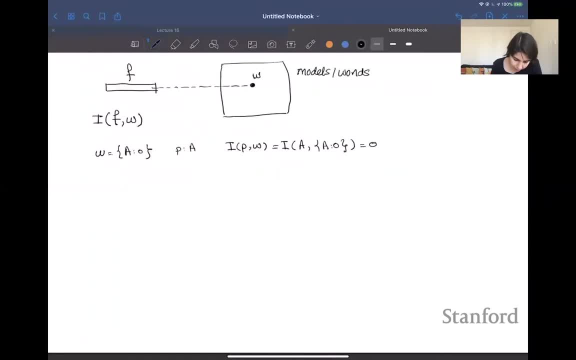 and I can check interpretation function of f and w. I can also be looking at a set of models right and I can call this models of f. And what is models of f right? Models of f is a setting where interpretation it's a set of w's, So let me write that here: models of f. what is that? equal? 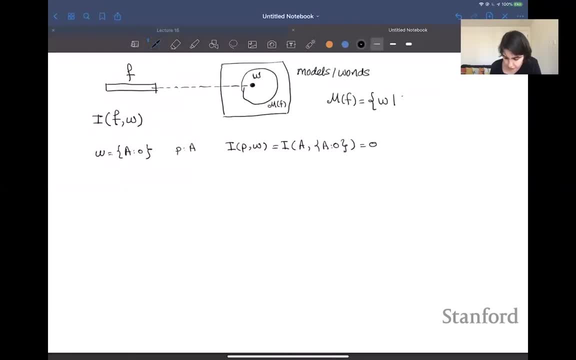 to. It's a set, it's a set of w's such that interpretation function of f and w is going to be equal to one. okay, So let me write that in the set of my definition. So we talked about interpretation function, we talked about a single model, and I don't know. 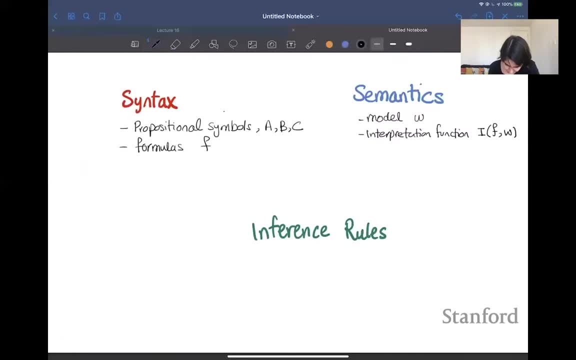 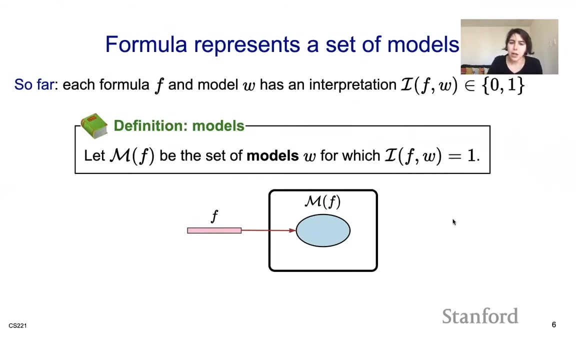 why this? does this erase this? We have models m of f. okay, And what is that? That is a set of w's, such that interpretation function of f and w is just equal to one. okay, All right. so now we have our models, Let's go back here, okay, All right. 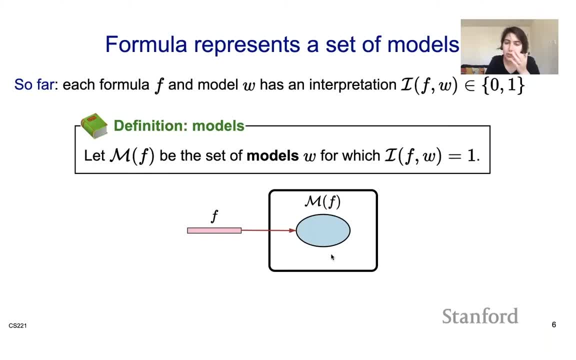 so basically, intuitively, you can think of this models of f as all the worlds, all the assignments where f holds, And anything outside of this is still like has some world, has some possibility, but that's a setting where this particular f doesn't necessarily hold. okay, So let's look. 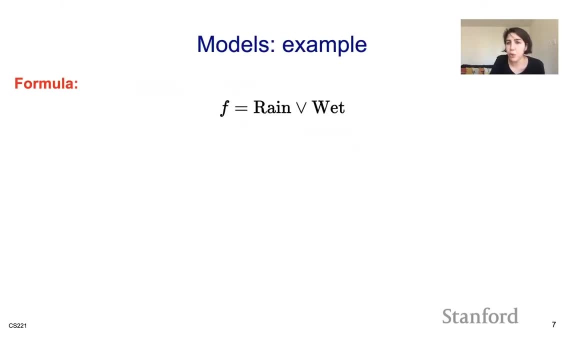 at an example. Let's say our formula f is rain or wet. okay, So then, if I think about models, all possible models are when we think about rain taking value zero or one and wet taking value zero or one. So I can kind of like show that by this two by two grid, That's all possible models. But what is models of? 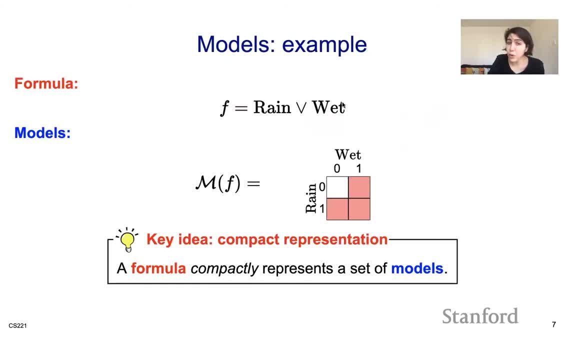 f. Models of f is when rain or wet holds, and that is the shaded area right. So the shaded area here is showing kind of like meaning of this formula. f, which is again symbolically written, doesn't have a meaning, but models of f is assigning a meaning to it. so it's saying, hey, these grids is showing like what? 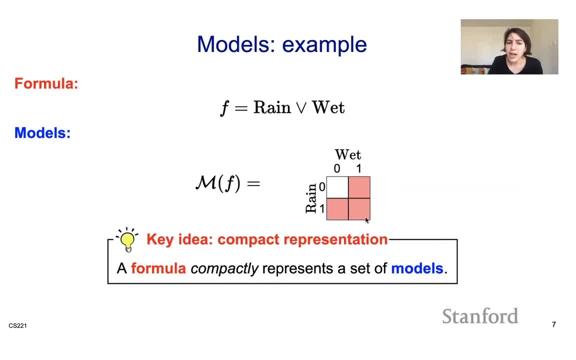 what is the meaning of rain or wet? okay, and, and the key idea here in logic in general is there's this formula: although it is written like again, syntactically, and it is- it is a symbolic representation, it's a very compact, like representation of a giant set of models, right, 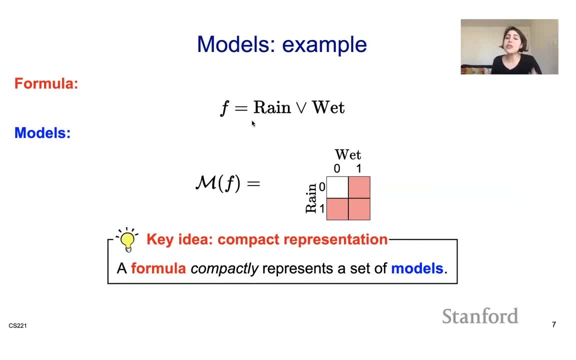 so. so in general, the nice thing about logic is is we could use formulas to compactly represent like, very like large meanings, like a lot of times like exponential meanings could be represented by, by formulas that are pretty compact and nice, and then that is kind of the power of logic. you. 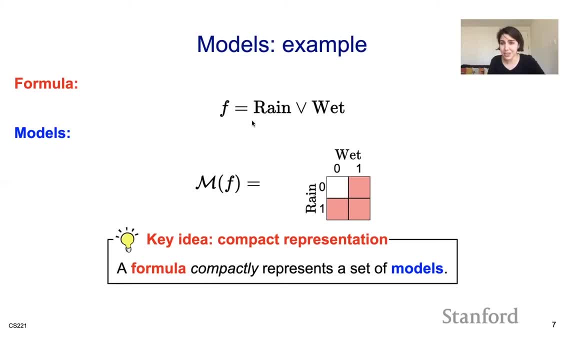 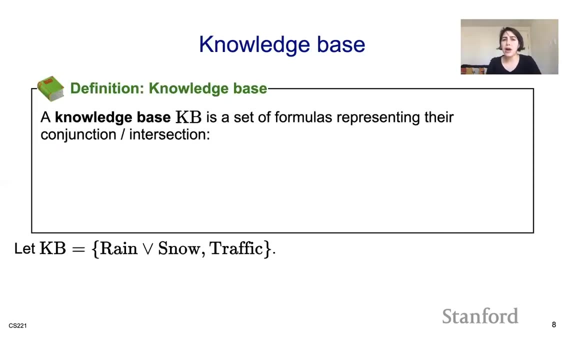 can write this compactly and you can do operations on it, you can do inference on it and so on, and and that that is really nice. okay, all right, so that was formulas and models and interpretation functions, binding formulas and models, you and, and what now we want to do, is you want to think about how could we do operations here and 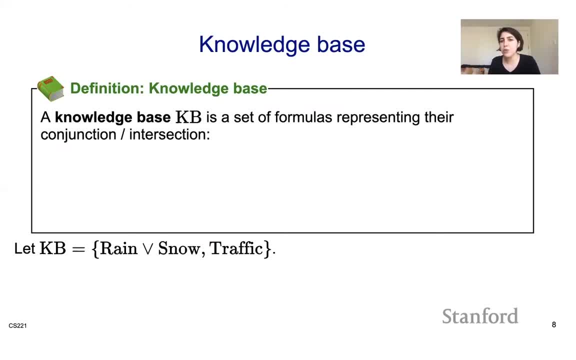 how could we what? what would? what would meanings like? what would new formulas add, in terms of meanings, to the knowledge that we already have? so for that, let's define something that's called a knowledge base. so a knowledge base is a set of formulas that i already know. okay, so if i have 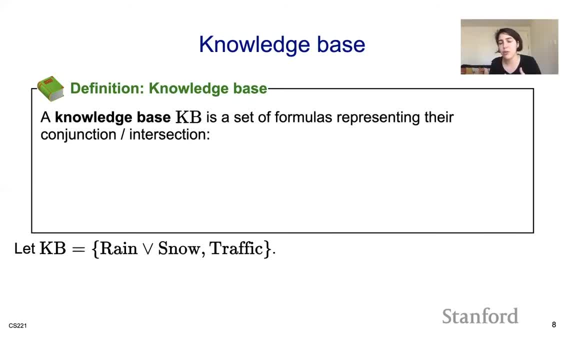 like a system, a virtual assistant system, that that i want to. i want to add logic to it or i want to speak to it using using language or using logic. that that system has a knowledge base and a performative result in operation. oriented on the model Java, we might use some kinds of. 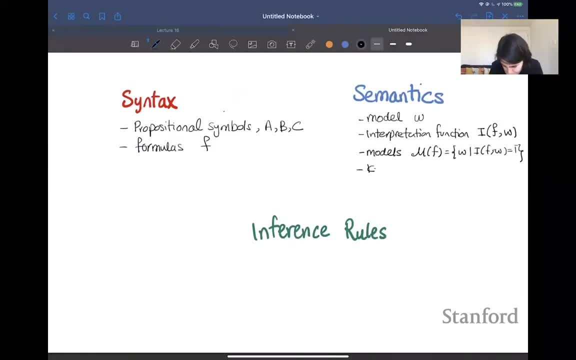 like x and an x that'd be like x. now you need to define plot starting point right and like the way we do. project strategy is by working more in the classroom. the holistically like in the class we follow, the farthestBonob closer to the solution and this is called a knowledge. 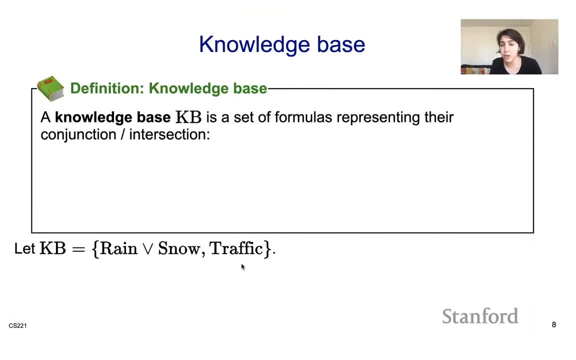 base, which is a set of formulas that are already represented, says rain or snow, or we might already know there's traffic. So this is our knowledge base. So then what happens is that someone might come and give me a new formula, and what we're interested in looking at is: how does that affect our knowledge base? 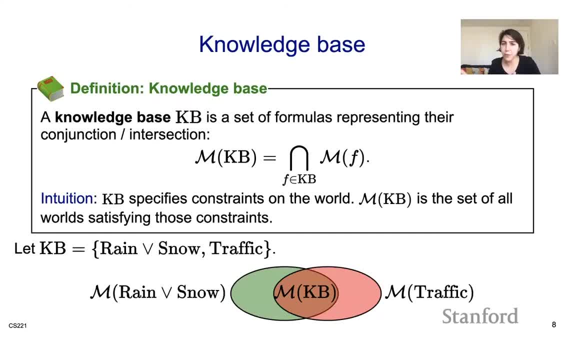 So before getting in there. so knowledge base is a set of formulas, so it is in the syntax land. What would be the analog of it in the semantics land? It would be models of kb. and what is the models of kb? Models of kb is going to be an intersection of models of f, So maybe let's go. 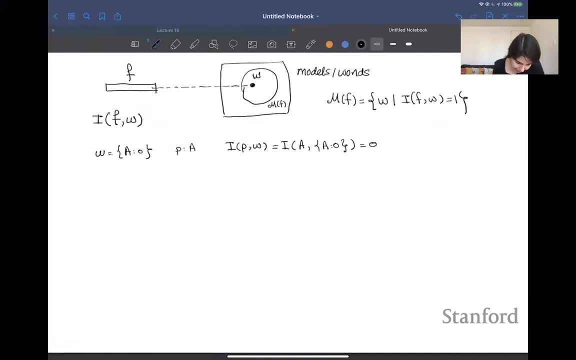 back here. Let me just look at an example. So we looked at an example where, let's say, I have a formula f1, and f1 says it's raining and snowing, And maybe I have f2, and f2 says there is traffic. Let me separate this. 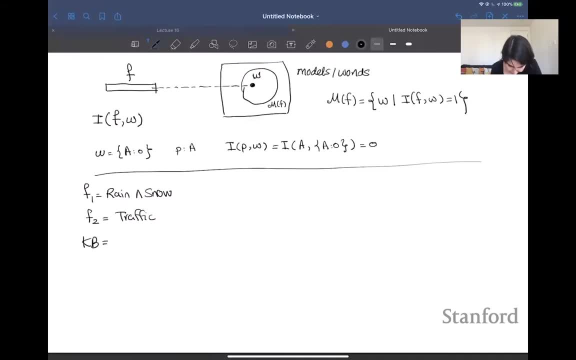 And I have a knowledge base, and my knowledge base has f1 and f2 in it. So someone already told me there's raining and snowing and then there's traffic, So what would be models of kb? So models of kb is going to be an intersection of models of f1 with models of f2.. And why is that? Because 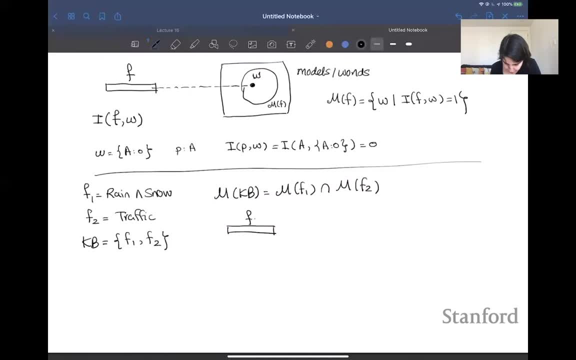 if you think about it, f1 is a formula, f1 has a set of models corresponding to it, models of f1 corresponding to it, And f2 is another formula that I'm just adding to my knowledge base And that has a bunch of other models corresponding to it And my knowledge base. 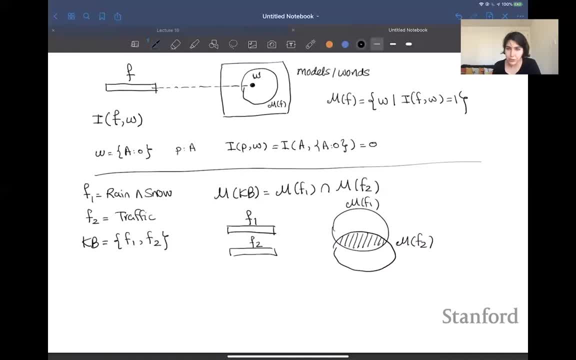 is now going to be an intersection of these two, Because as we add more formulas, as we add more knowledge to our knowledge base, then our models is going to become smaller and smaller because we are adding more constraints, which is pretty interesting. So, in general, if I have let me, 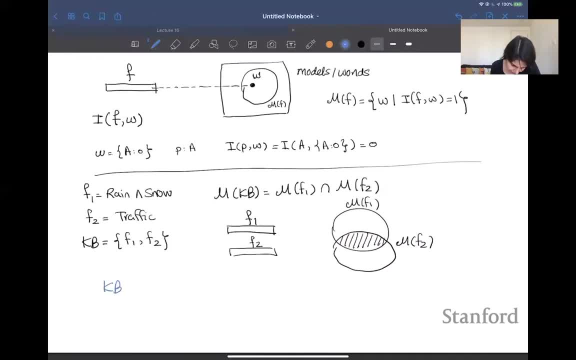 write that in a different color. So if I have a knowledge base and I add a new formula to that knowledge base- maybe a union with a new formula that is added f, what would be the effect of that on models of kb? The effect of that on models of kb is going to be what I had for models of kb. 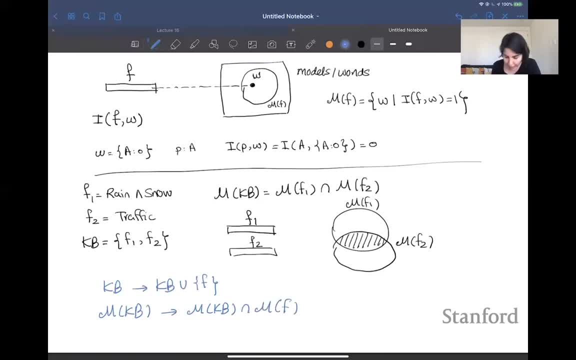 intersection models of that. So adding new formulas is constraining our models, constraining the meaning more and more, Because it can be like if you have raining and snowing and we have traffic as a whole, other set of models, the intersection of the two. 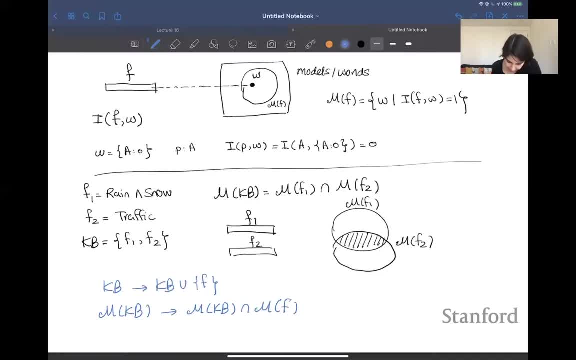 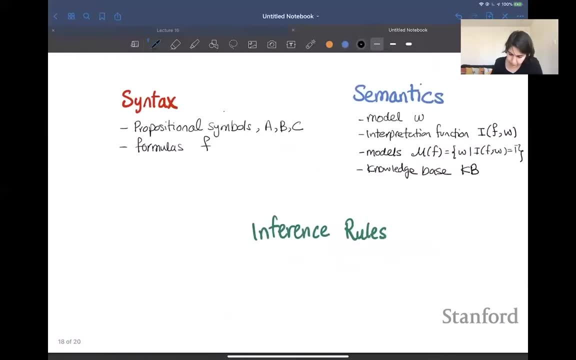 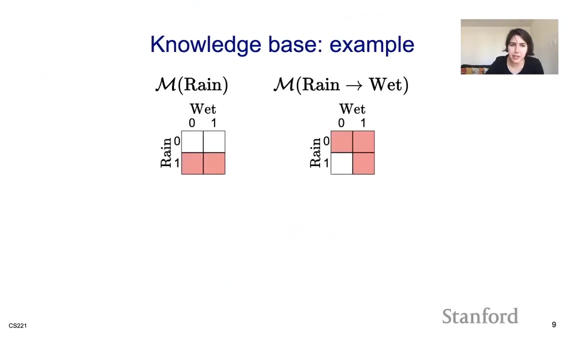 is going to give me this models, So also let me connect this. So this corresponds to these models. this corresponds to these models. All right, So let's go back here. So that's how we define models of knowledge base. Let's look at another example here. 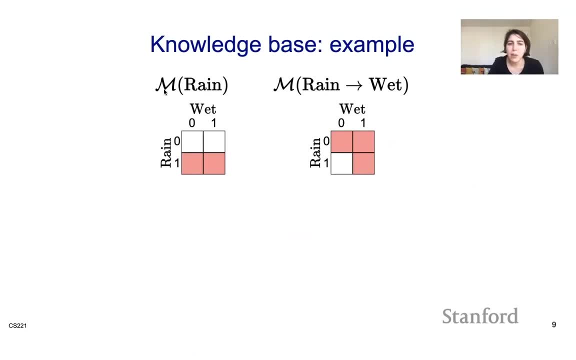 So let's say we're looking at the raining as one formula. models of rain is going to be this shaded area where rain is equal to one. And then we have another formula: Rain implies wet. And what is? models of rain implies wet? It is basically the negation of rain or wet. 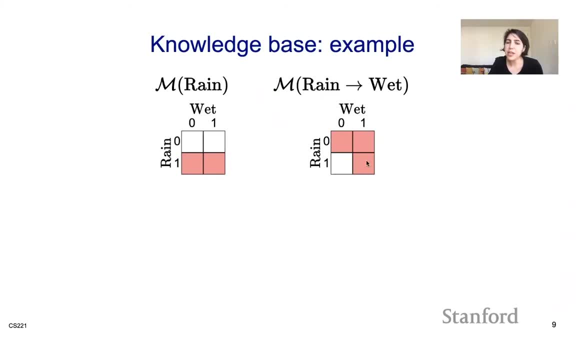 So basically, it's this shaded area. If I'm looking at a knowledge base that has both of these in it, then what would be the models of that model? knowledge base is just going to be the intersection of these two shaded area, which is basically this. 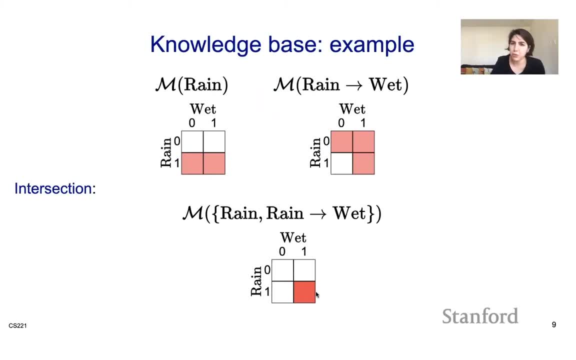 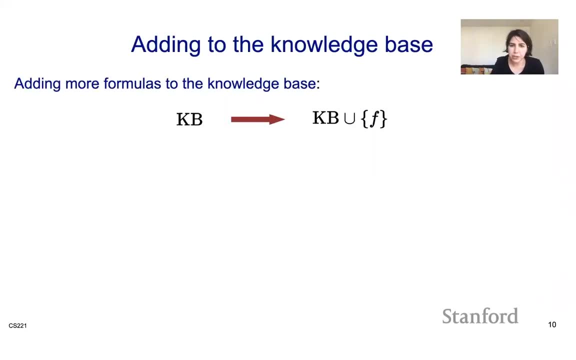 square okay, where we have both rain, and rain implies rent folding. All right, sounds good. And then- this is what I've already basically mentioned- We have knowledge base. If we add a formula to it, it increases the size of our knowledge base. We are shrinking the size of. 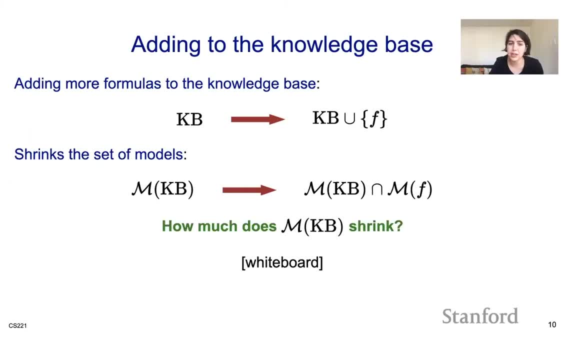 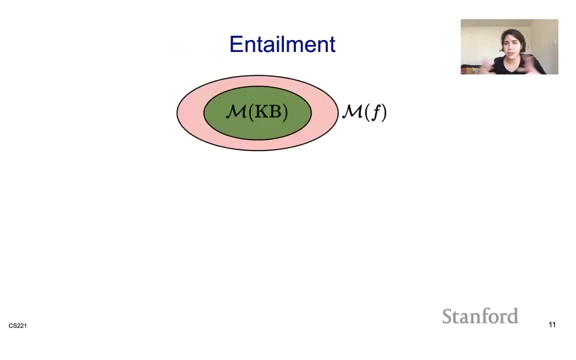 set of models because we are constraining things more and more. So we are constraining the meaning part. All right, so now let's talk about this idea of what happens if I have a knowledge base and I add a new formula. So I have a knowledge base, I'm trying to add a new formula. see what? 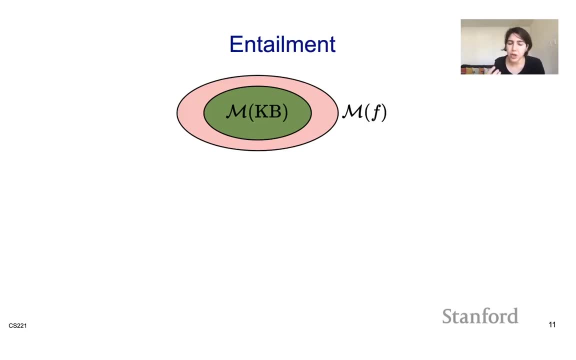 happens, And there are three things that can happen. So one option is entailment. So what entailment says is: if I have a knowledge base, if I have KB as my knowledge base, and you come and tell me a new formula F and that formula is not adding anything to my knowledge base, then we say: 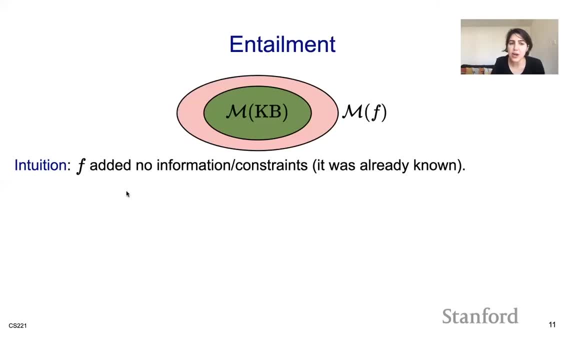 we have entailment. So this is a scenario where F is just not adding any information or any new constraints. This is basically telling me things I already knew. So we say KB entails F and that is written using this double line kind of symbol. So we say KB entails F if, and only if, models of 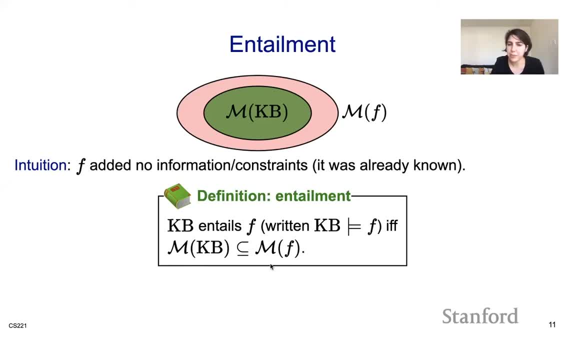 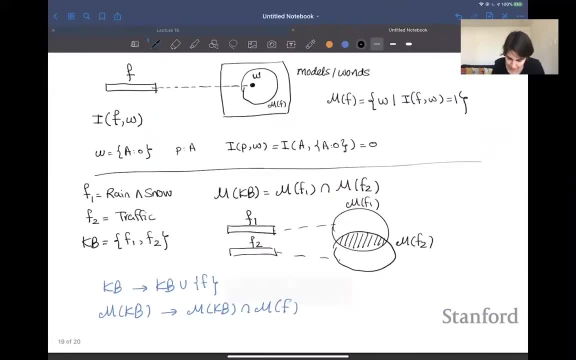 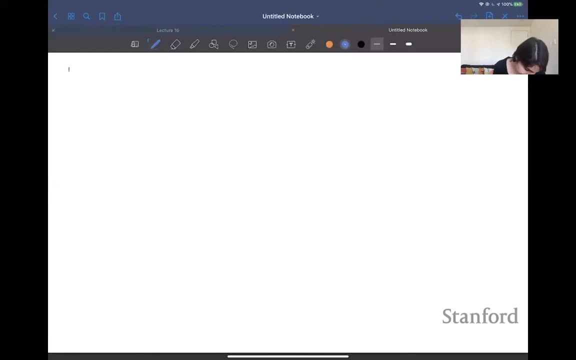 KB is an intersection of models of F. Let's look at an example here. So let's go back to the formula. Let's go back here. Maybe I'll start anew. So we have three options. One is called entailment- Entailment, Yeah. So let's start with a knowledge base, And my knowledge base, maybe, is: 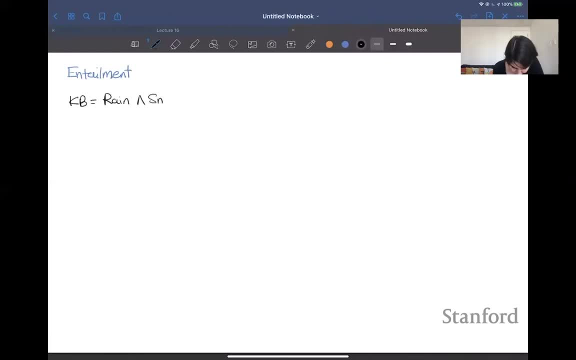 rain and snow. So I have a formula in my knowledge base that says rain and snow And that has models corresponding to it. So this is models of KB, And you might come and tell me a new formula, and that new formula is rain. And if you tell me rain, and I already have rain and snow in my 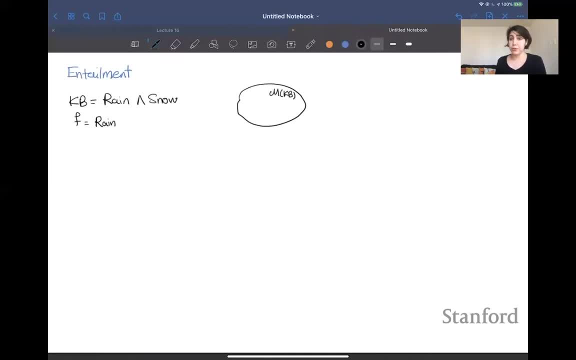 knowledge base. that doesn't add any knowledge to me, right, Like I already knew, it was raining. So then this models is going to be a super models of F, is going to be a superset of models of KB. Okay, so we say KB entails F if, and only if, models of KB is an intersection of models of F. 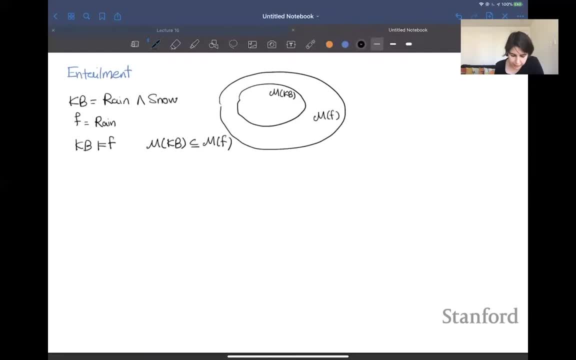 So didn't tell me anything new, already knew that. and that is entailment, So let me go back here and maybe add these under our definition. So now we have defined entailment in terms of models of KB, So let me go back here and maybe add these under our definition. 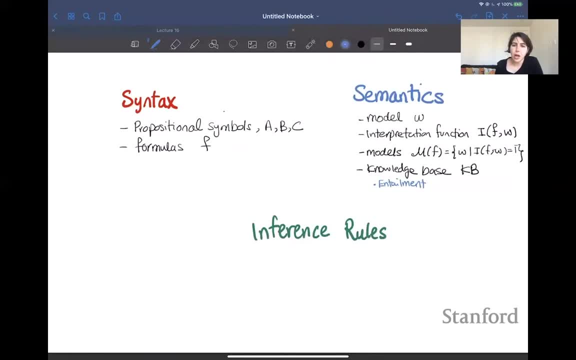 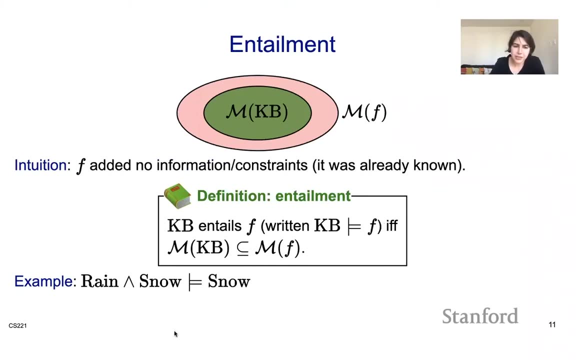 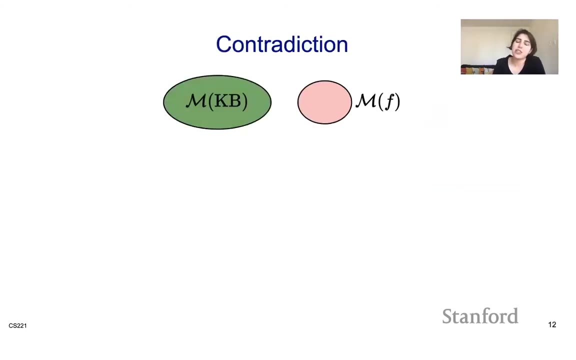 Okay, all right, So let's go back here. So rain and snow is entailing snow. So okay, so that was one option. Another option is contradiction. So what is contradiction? Contradiction is a scenario where you're telling me a new formula F. I already have a knowledge. 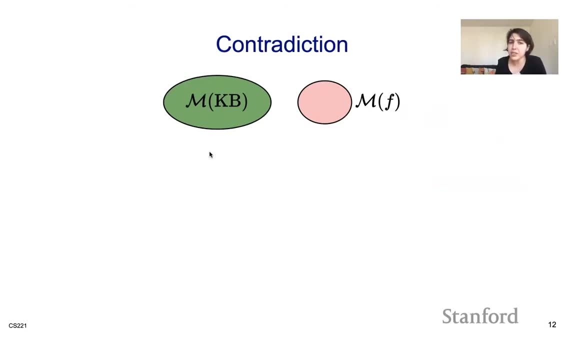 base KB. you tell me a new formula, F, and that is contradicting with my knowledge base. okay, So in the models land, what happens is that models of KB doesn't have any intersections with models of F. okay, So F contradicts what we know, our knowledge base if, and only if, models of KB. 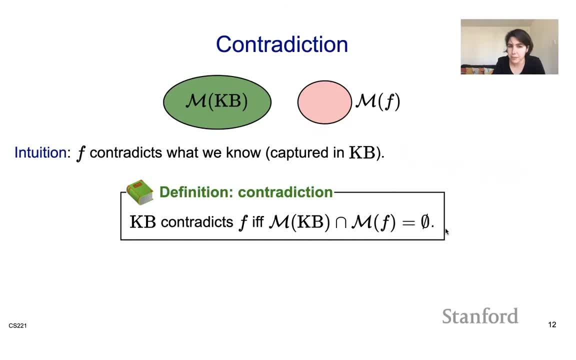 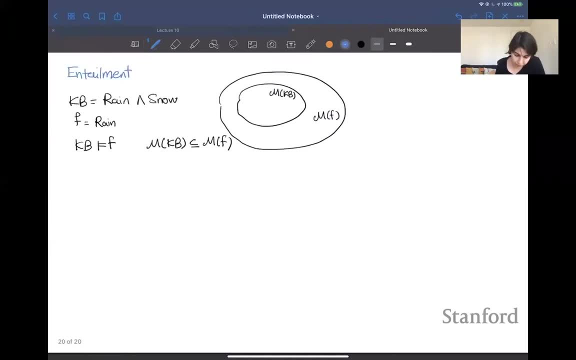 intersection models of F is going to be the antiseptic right. So let's look at an example, Let's maybe go back here. So our second option is contradiction. So let's write that here: Contradiction. So contradiction is a scenario where I know some knowledge base. So my knowledge, 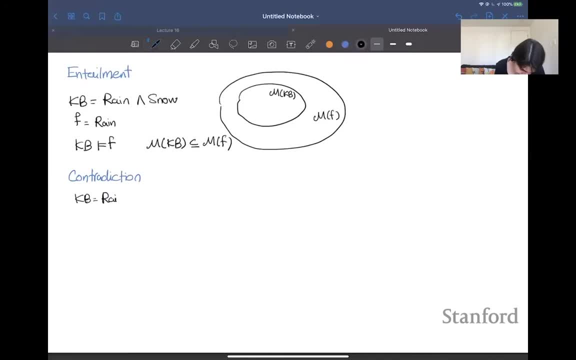 base is maybe rain and snow again. So I think it's raining and snowing, And then you come and tell me a new formula, and that new formula is negation of snow, maybe okay, And then that contradicts with my knowledge base, right? So if that contradicts with my knowledge base, 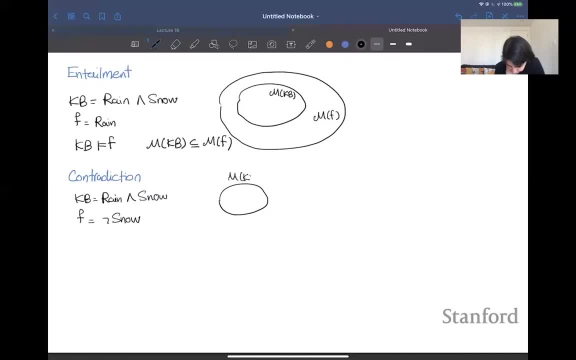 what happens is that there is a models of KB and there is a models of F and they don't have any intersection. So contradiction is a scenario where models of KB intersection models of F is empty, okay. One other interesting thing to kind of like notice here is that if you think about 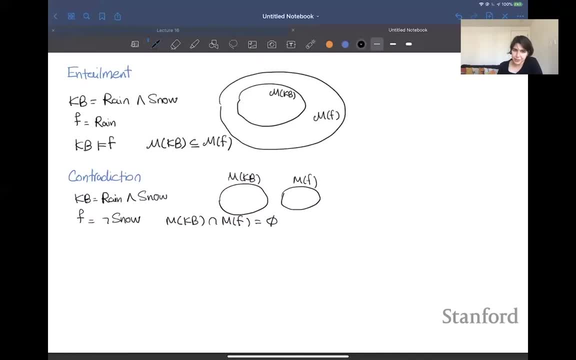 contradiction. contradiction is very related to entailment. Contradiction is the same thing as entailing negation of F. And why is that the case? Because if you look at models of F- right Models of negation of F- is anything outside of it right? 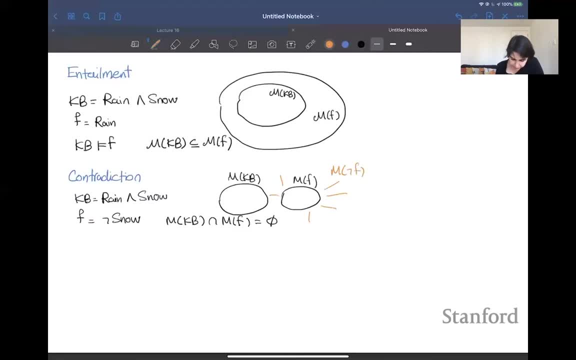 So if this is models of negation of F, then what is happening? The thing that's happening is that models of KB is a subset of models of negation of F And if you remember our definition of entailment, that is the same thing as KB. 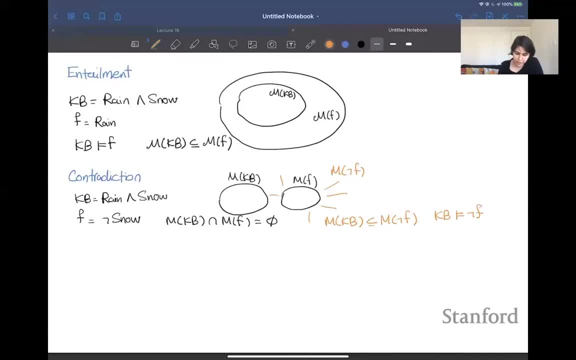 Entailing negation of F. So that's pretty interesting, because contradiction is the same thing as entailing negation of F. All right, So those were the two cases so far. right, You either tell me a new formula- and I already knew it, so that is entailment- or you tell me: 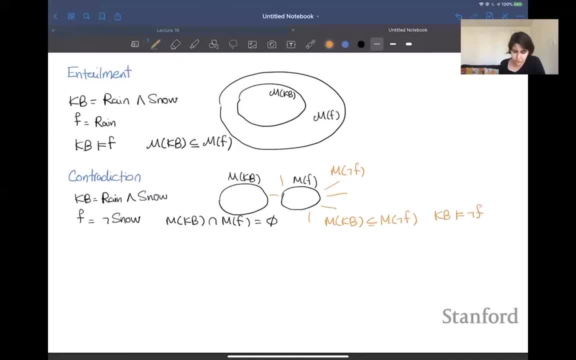 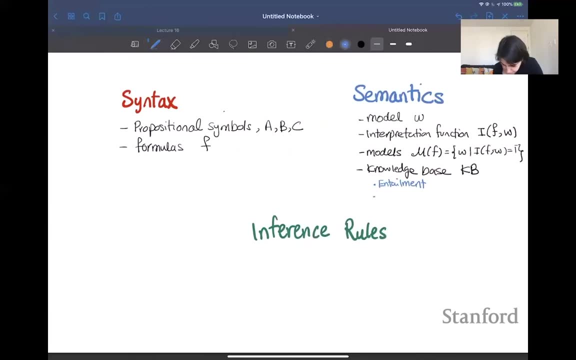 a new formula and that contradicts the knowledge base that I've had. so that is contradiction. Okay, And let's add that here. So we talked about entailment. Now we've talked About contradiction, And we wrote entailment as KB entailing a formula, and contradiction is KB entailing negation. 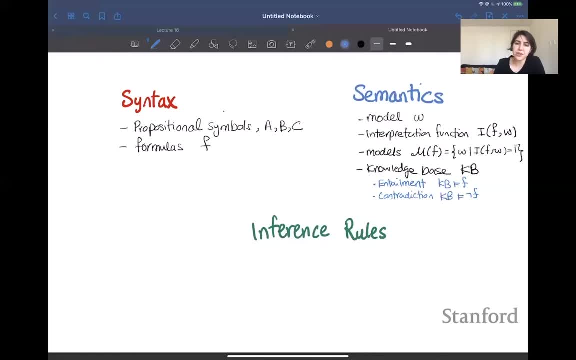 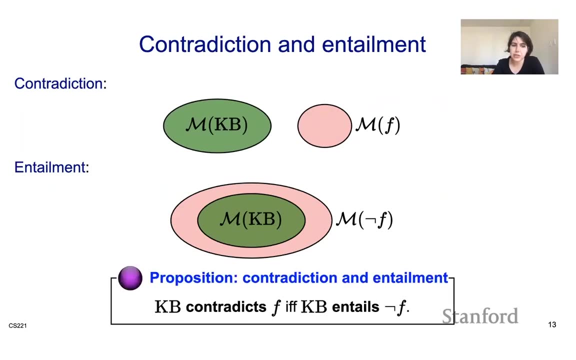 of a formula. All right, So there is a third case. Let's talk about that third case. Let me skip that. So we talked about contradiction being very related to entailment, and KB contradicting with F is the same thing as KB entailing negation of F. 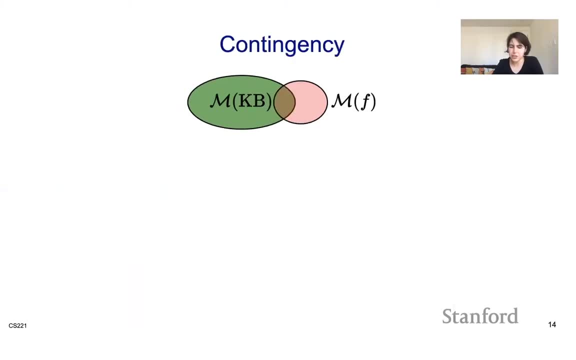 All right. So the third case here is what we're calling contingency, And that is when you are telling me a formula. That formula is adding is actually telling you something I didn't know. It's telling me some non-trivial information. Okay so. 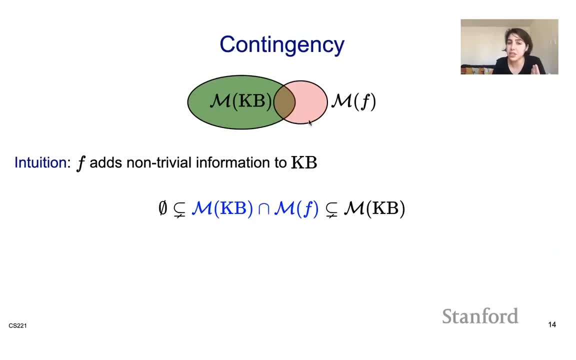 So that is when models of KB has some intersection, some non-trivial intersection with models. So so that is when we write models of KB intersection models of F. is is going to be a subset of models of KB, but it's going to be strictly. 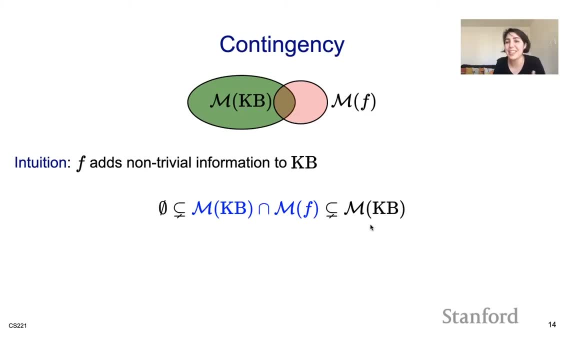 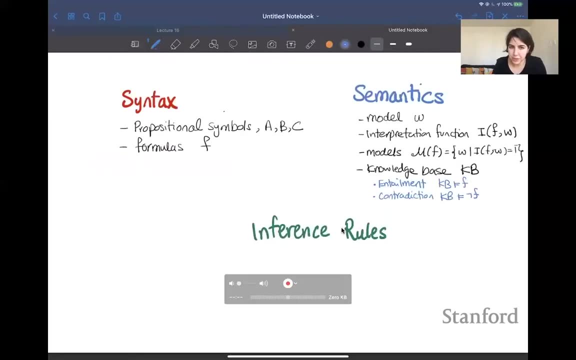 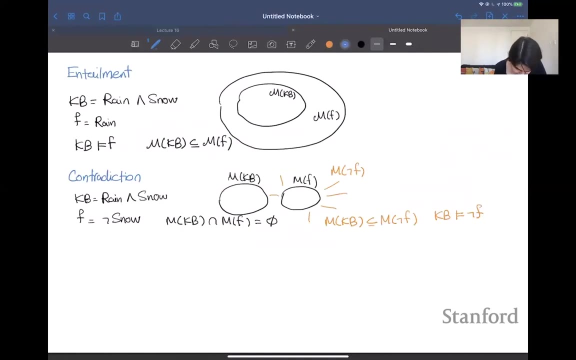 subset of models of kb. if this is equal, like we get entailment, so we don't include equality here. all right, let's look at an example, maybe. um, let's go back here. so our third case is contingency, and that is when i have maybe my knowledge base and maybe my knowledge base is just. 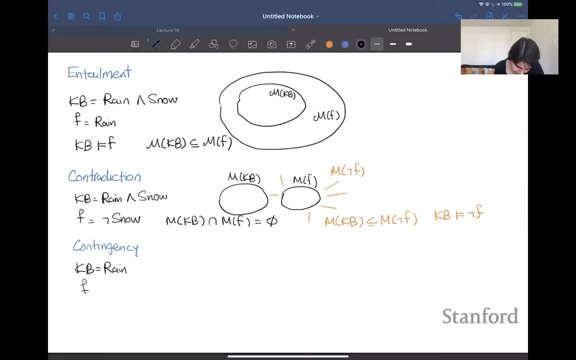 rain this time, and you come and tell me a new formula, and that new formula is snow. okay, so so my knowledge base thought it is raining, so i have my models of knowledge base corresponding to raining here, and then you come and tell me: hey, by the way it is, it is also snowing. 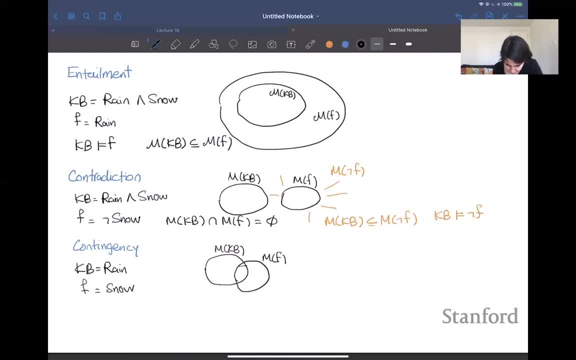 and models of snowing is here and there is some non-trivial intersection going on here. okay, so. so contingency is when models of kb intersection. models of f is going to be a subset and it's not going to be equal to models of kb and similarly, empty set is going to. 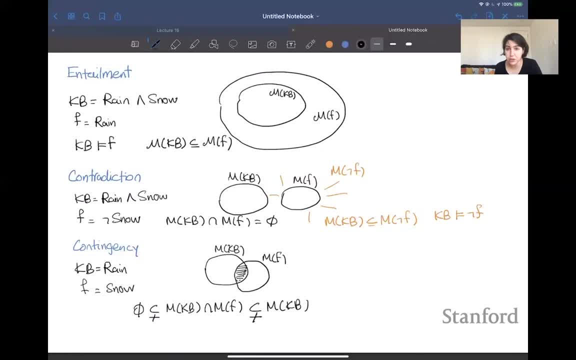 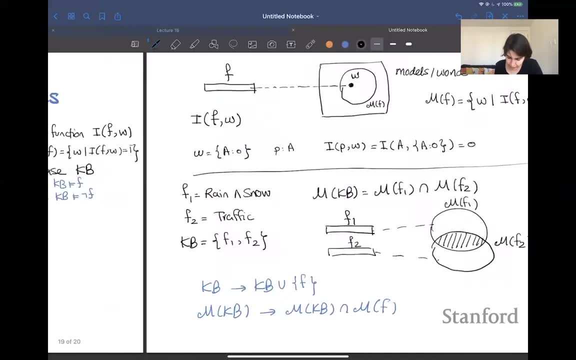 be a subset of this, but it's not going to be equal. so if you get like some non-trivial information, something that you didn't know, and that gets added, okay. so so that is contingency. and, going back here, let me add contingency as the third option. 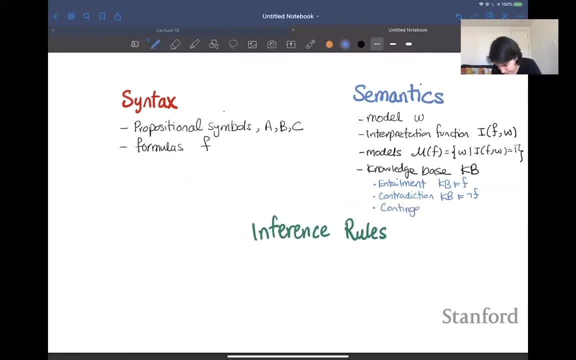 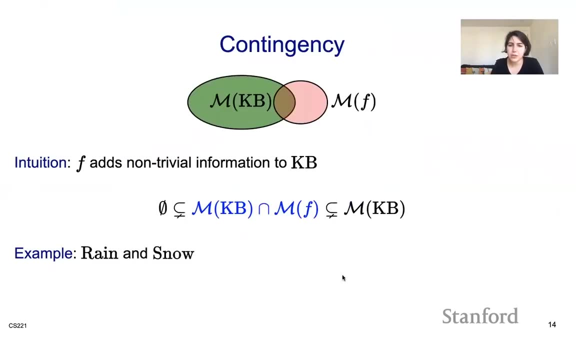 contingency and contingency. um, as, when you have these non-trivial intersections, i'm not gonna write it out. all right, let's go back here, okay, so? so we have these three possibilities. you give me a new formula. i'm either entailing it or contradicting it, or or i have contingency. so now let's talk about. 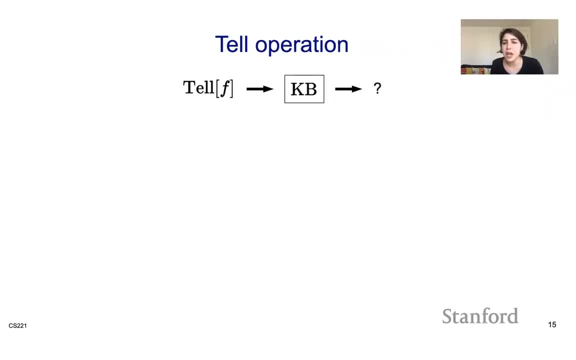 let's talk about how we would use these ideas if we want to implement a virtual assistant. remember like we started this lecture thinking about having a virtual assistant where we can talk to it in logic or language, and that gives us something that gives us a little of our application in terms of. 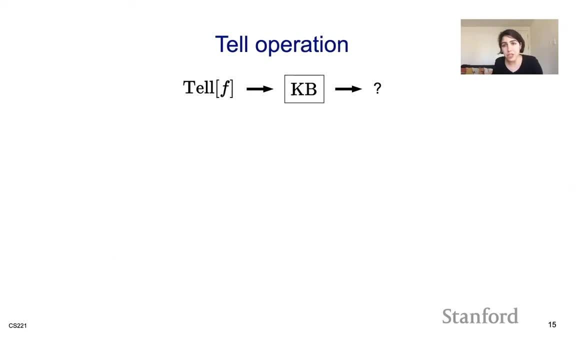 And that virtual assistance, right, like you can tell it some information or we can ask it questions, And then maybe you want to implement this tell operation. So if I want to implement a tell operation in this, in this virtual assistance, this virtual assistance is going to have some knowledge base- at the moment some KD- And I tell it: F, a new formula, F. So what can happen? So if I tell it a new formula, maybe I tell it it is raining, So I do tell rain- three things can happen, right, 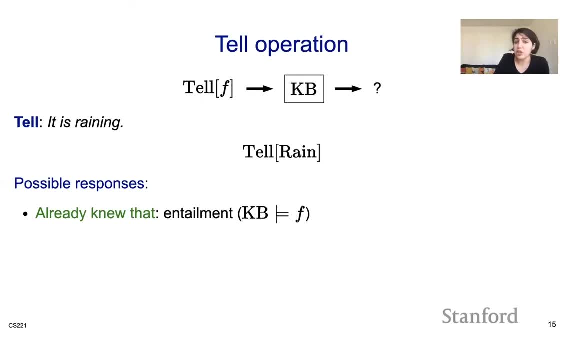 It can either. it can either entail F right, my knowledge base might already like have raining in it. In that case, the response to tell operation, tell, tell it is raining, it's going to be. I already knew that. Okay, so so if it says if my virtual assistant already entails rain, it should respond to me, as I already knew that. 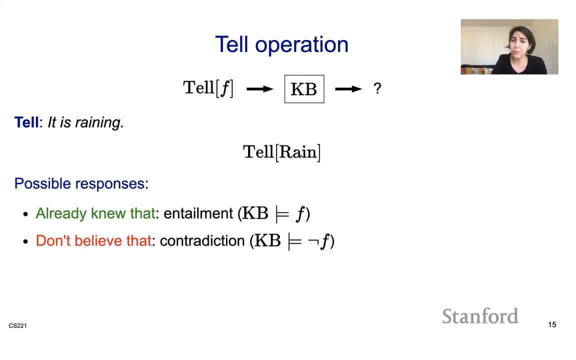 Okay. if it contradicts that, it should say: I don't believe that because it's knowledge base basically says it's not raining And now you're telling it it is raining And because of that it would respond as I don't believe that because my knowledge base tells me the opposite. 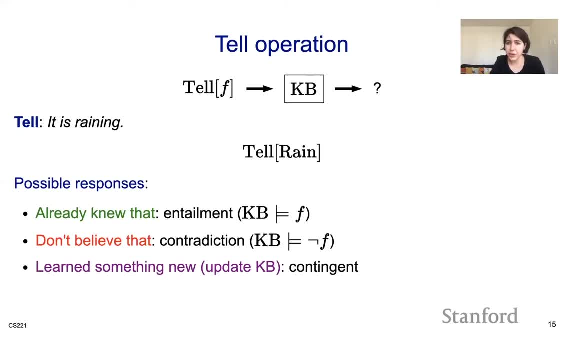 Or if you're telling it something new, you're telling it it is raining and it didn't know that or didn't have any information about it, then it should say: I learned something new. And, based on that thing that you're telling it, it should update knowledge base, it should update its KB by by this, this new formula. 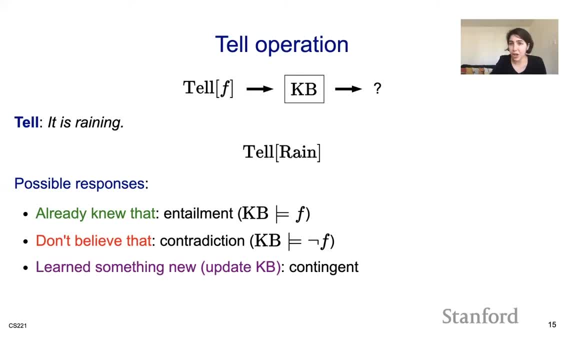 That it is raining, Okay, so? so now we can implement a tell operation based on, based on these three ideas of entailment, contingency and contradiction. In a very similar fashion, we can also implement an ask operation. If you ask it is it raining, then based on that, it can, it can go ahead and it can answer yes, a definite yes, if KB already entails F. So if you have entailment, it should answer no. if you have a contradiction, if KB contradicts F, right, or if KB entails F. 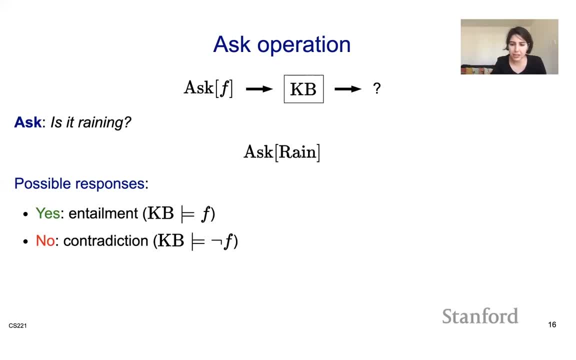 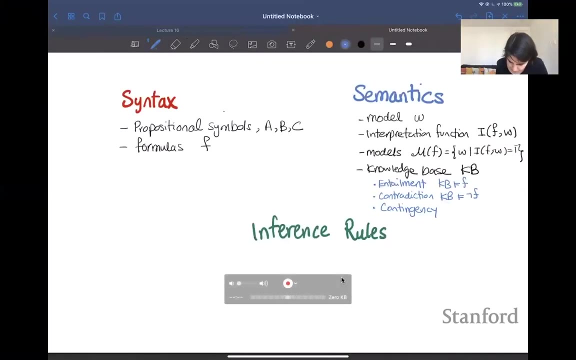 negation of F. So it should give us a definite no, no, that there is a contradiction. Or it should tell us: I don't know if there is contingency, it doesn't know. So if you ask it, is it raining? it doesn't know. So it should just say: I don't know. So so, going back to the things we were defining here, let me, let me move this inference rule thing. 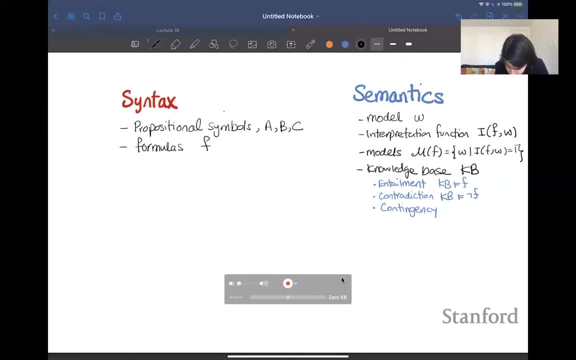 So, um, let me just write tell and so. so we talked about this tell and ask operation and we can basically say: okay, so let's say we have entailment, So we can basically implement tell and ask based on this entailment. contradiction and contingency. 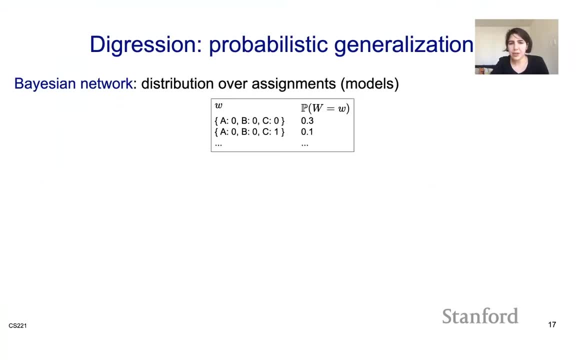 All right, so I want to just do a quick side note here. I don't want to go into this in too much detail, but there is a connection between the things we were talking about here and some of the topics we discussed, like two weeks ago in Bayesian networks, right? 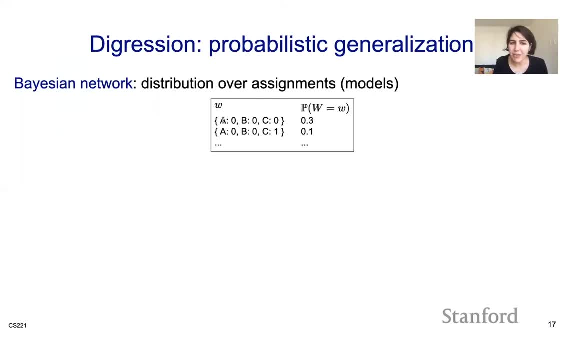 So so we've been talking about this idea of models and having having these types of these types of models, And this is the same thing as assignments, Right? And you can think of it. you can basically think of having Bayesian networks as a distribution over these assignments, over these models, Right? 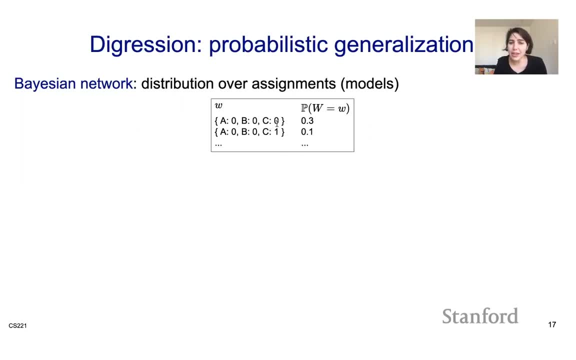 I can have like a equal to zero, b equal to zero, c equal to zero And I can have a probability assigned to that, like probability of that could be 0.3. or I can have another assignment or model and I can have another probability assigned to it. 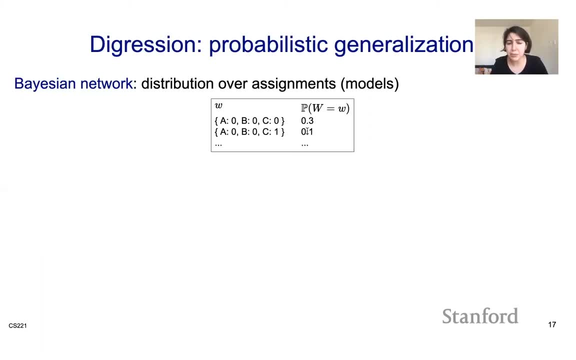 So from a Bayesian network perspective, from probabilistic perspective, one can think about logic in a probabilistic way And think about the probability of a formula given a knowledge base. So so when you have a knowledge base, you have some knowledge and and you're asking about a formula one can think of. instead of thinking about just these three different things like entailment, contradiction and contingency, one can think of a probability like an actual, like value, right? 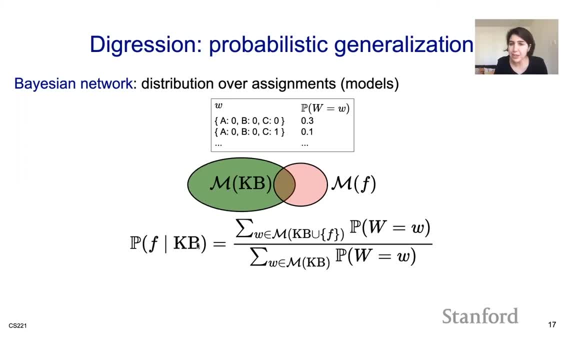 And probability of the formula given a knowledge base. so what is that going to be equal to? That is going to be equal to probability of models, double use, that that exists in the in the intersection of models, KB and models of that right over probability of all possible models and not knowledge base. So so double use are all possible models in my knowledge base. I'm going to sum over all those probabilities of all possible. 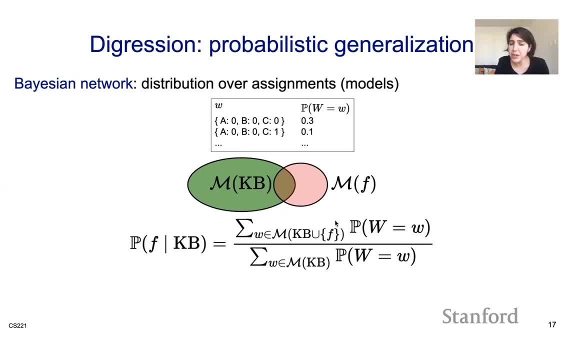 Models in my knowledge base, in the denominator and in the numerator. I'm going to just focus on models that are in the intersection of models of KB and models of that And then the union. So so models of KB, union F is equal to models of KB, intersection models of that. 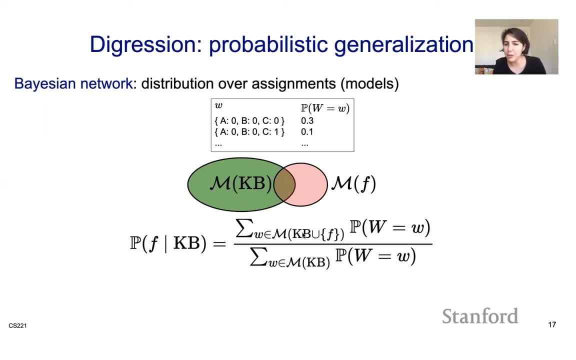 That's why there's a union here. You're, you remember, like if you add an F to your KB, you're shrinking your knowledge base. So, so that's why this, this numerator, is smaller, right, you're shrinking. you're shrinking your knowledge base by adding this F to it. 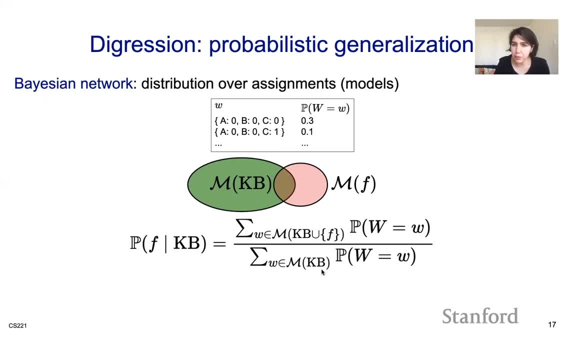 Okay, And if you think about this fraction, right, this is a number, This is a number between zero and one, And now we have probabilities. We have actually like a probability for F, like being satisfied or not given, given a knowledge base, But in general, like this was just like a quick digression, like talking about 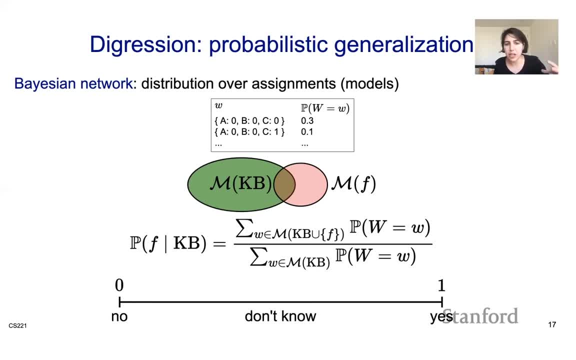 A probabilistic view of this. There's quite a bit of work actually in logic and probabilistic versions of it And thinking about probabilistic model checking and instead of giving just like zero one values, what would be a probabilistic view of it? 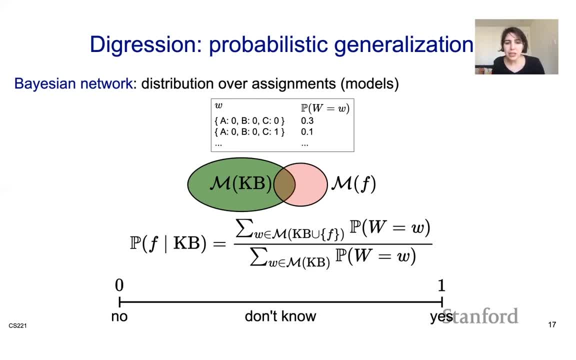 We're not going to go into details of those in this class and and basically you can think of these probabilities as these three different ways of looking at the problem that we've been talking about. if this probability is equal to zero, Then then we basically have an answer. No, we have contradiction, right like F is not. 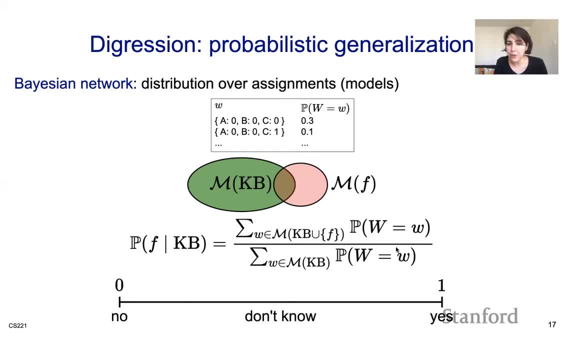 Satisfied. Well, if this probability is equal to one, if numerator and denominator equal to each other, then you're answering Yes, right, like F is not adding any information. So we have entailment. And if you get any other value between any other value between zero and one, then you're in an entailment situation. Sorry, we are in a sorry contingency situation and we basically say we don't know. right, like any of them, We basically say we don't know. 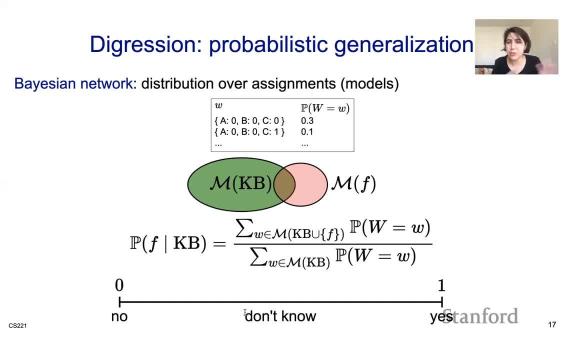 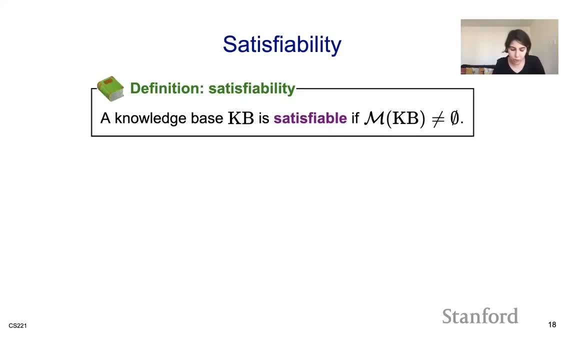 Alright, so so that was just a quick kind of like connection to The probabilistic generalization of some of the things you're talking about, an invasion networks. But now let's just go back to go back to the same problem you're talking about. 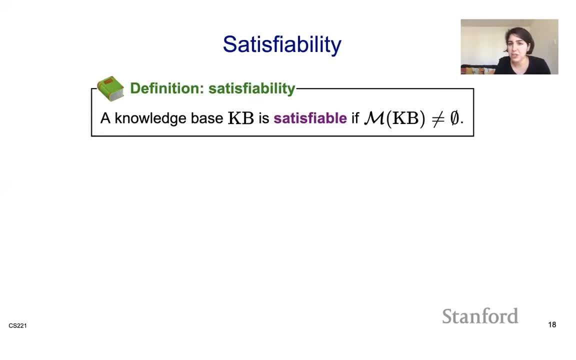 Right. So so we've talked about these three different things entailment, contingency and contradiction. We've talked about how we can have a tell and ask, operate operator based on that. Now we're going to talk about this idea of satisfiability. So what is satisfiability? So a knowledge base, KB is satisfiable if models of KB is not empty. 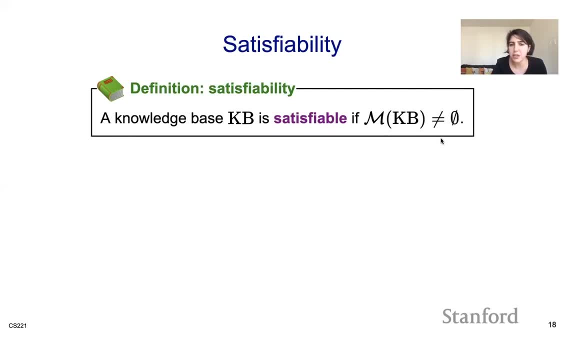 Okay, very simple. like: not models of KB is not empty. We have satisfiable. So why is satisfiability useful? Why am I talking about this as satisfiability? because satisfiability is a well known problem. We have really good like solvers for it: SAT solvers. 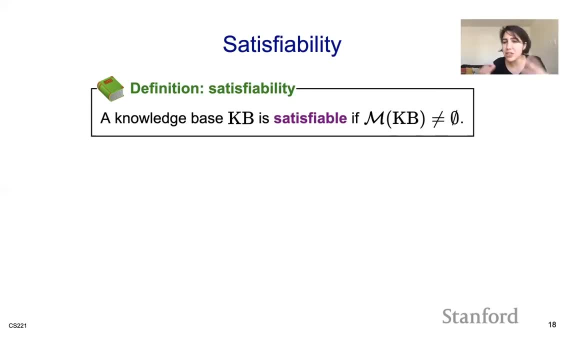 And then we're going to talk about that in one slide really quickly. So it's nice to think about these three different things: entailment and contingency and and contradiction, In kind of a view of a problem of satisfiability. Okay, so so we have these three things. satisfiability gives me a yes or no answer. So how can I use satisfiability to answer if you're in either in any of these situations? 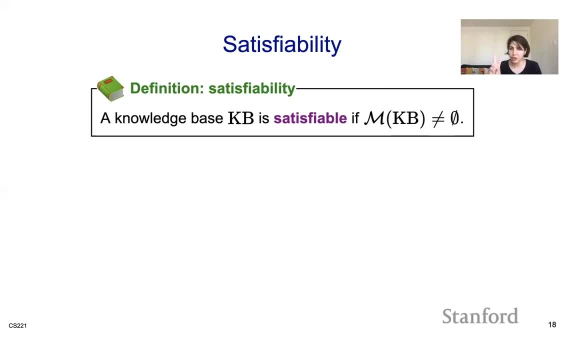 So so the radio satisfiability is we do two calls to satisfy ability. So The first call is in general if I want to think about my ask operator or tell operator, and if I want to reduce it to satisfy ability, I can. I can do two calls to satisfy ability. I can first ask. 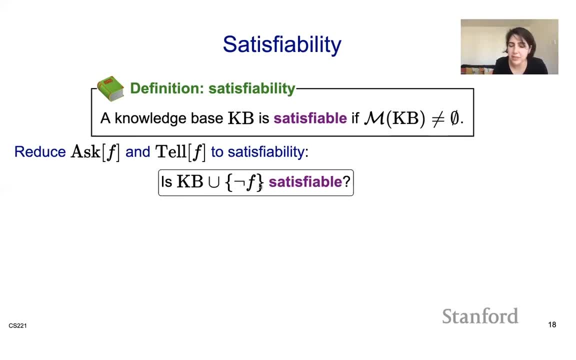 If KB you need to, Negation of a is satisfiable or not, Okay, so what does the answer to that give me? So if I get no for that right, if KB you need, a, negation of F is not satisfiable, I have entailment right. so I get my my answer for entailment here. 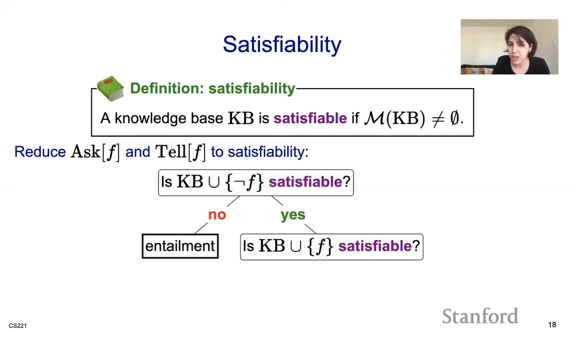 And if I get yes for that, that doesn't answer everything right, like if I just get yes for this, I don't know if I'm in a contingency situation or contradiction situation. So what do I need to do? I need to do another call to satisfiable 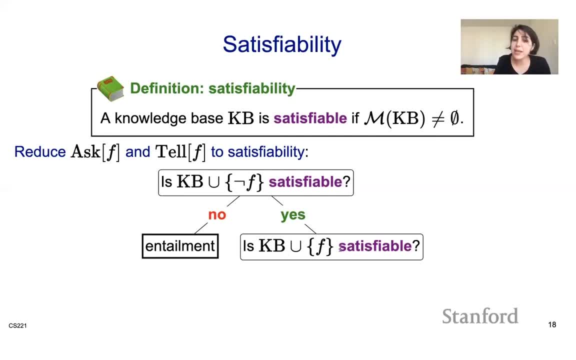 And the second call to satisfy Ability is asking if KB you need an F is satisfiable. And what does that check? Well, well, if I get no for that, then I'm getting contradiction. Remember, contradiction is the same thing as entailing negation of F. 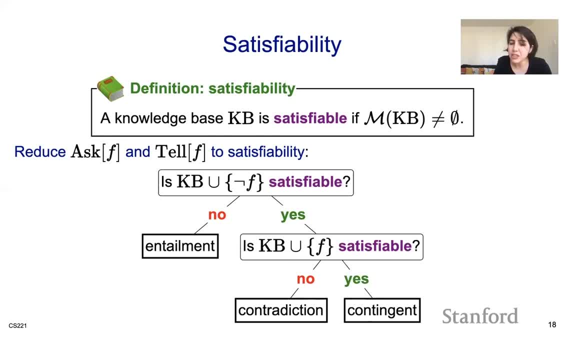 That is why the answer for this gives me contradiction, And if I get yes for that, I get contingency. So what I've just done is is if I in general, if I want to know if I'm in the entailment contradiction or contingency situation, then I can basically figure that out with two calls to satisfiable. 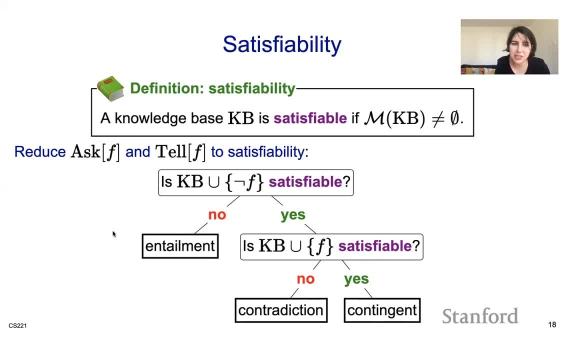 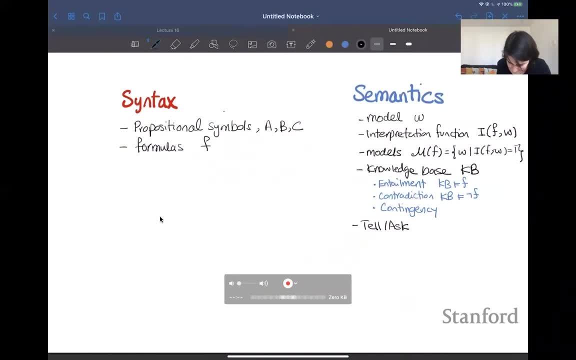 And why do I want to know if I'm in any of these situations? because that helps me implement my ask until operations. So going back here. So we talked about ask until we talked about how it relates to entailing contradiction and contingency, And now we have talked about satisfiability as a way of answering which scenario we are in. 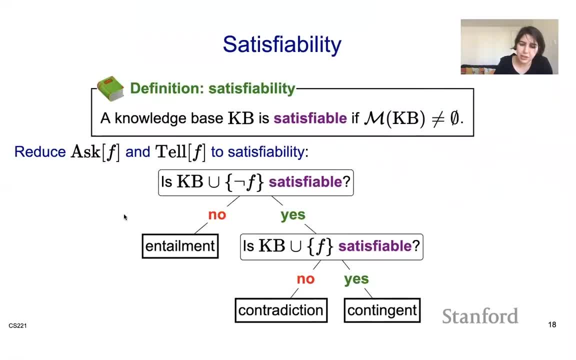 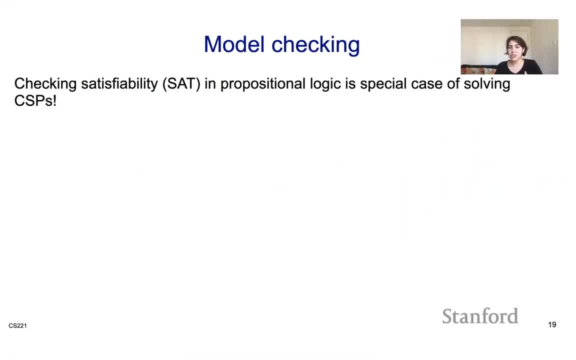 And how we answer satisfiability. So. so that's a good question to ask. So what is satisfiability? So satisfiability In checking satisfiability? the SAT problem in propositional logic is basically just a special case of solving a constraint. satisfaction problem is CSP. 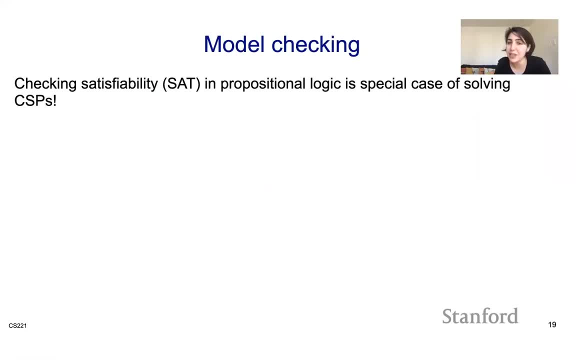 And we have already like, like, learned about CSPs and solving CSPs. So what that means is we can basically check satisfiability. we can basically Check, check if the CSP problem, like what's the solution to the CSP problem- and solve satisfiability with algorithms that we already have access to. 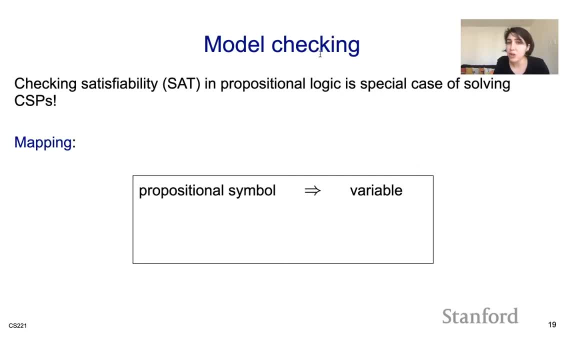 And this idea Of checking satisfiability is called model checking. you're checking if a model exists or not. you're checking if an assignment exists or not. Okay, so so the mapping of the SAT problem to CSPs is as follows. So propositional symbols are basically variables, what we used to call variables. 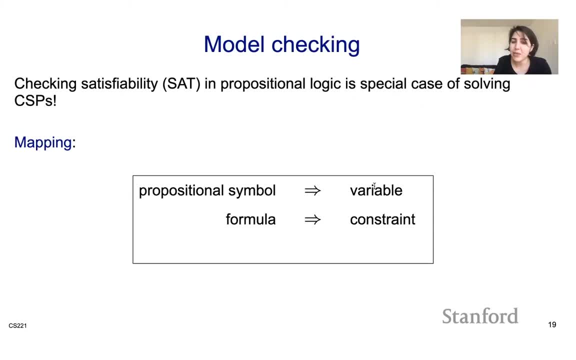 formulas are basically constraints And then, if you have variables and constraints, you can come up with an assignment and that assignment is basically a model. So you're checking if a model exists or not. You're checking if it's, If it's satisfying assignment exists or not. 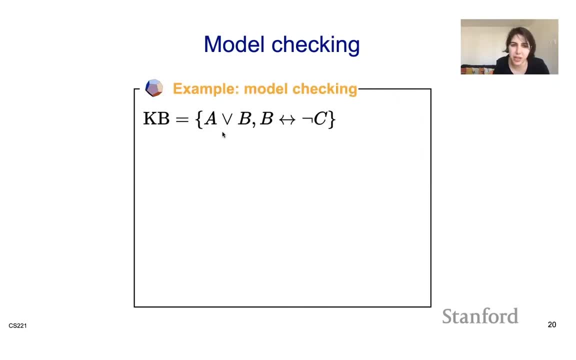 Let's look at an example. So let's say our knowledge base has these two formulas in it. We have A or B and we have B- bidirectional implication, negation of C. Alright, so we have three symbols: A, B and C. These symbols are the same things as CSP variables. So we can have three nodes, these three variables. 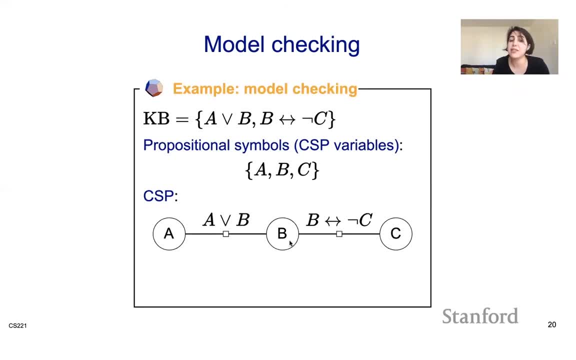 And then we have basically two formulas. These formulas create constraints In our CSP. So we have A or B, and then we have. we have B, equivalent negation of C. And then what are we doing? So we have a CSP. we can solve it right. we can find an assignment, a consistent assignment for it, which is the same thing as a satisfying model. 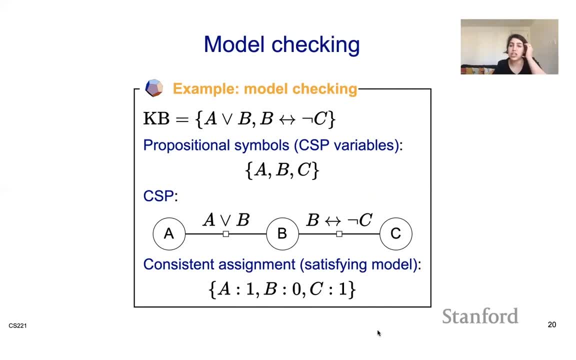 And if you find an assignment, This problem is satisfied. Well, model checking comes up with a model for it. And then, if it is not satisfied, Well, it's going to return as unsat. It doesn't come up with any assignments. 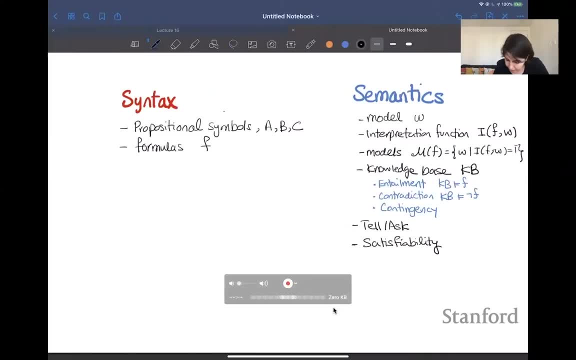 So so that's kind of nice going back here right like this problem That we've been talking about. this tell and ask operation reduces to entailment, contradiction and contingency. I can use satisfiability- two calls to satisfiability to- to answer that. Then how do I do that? Well, I use model checkers to do that, So so that's called model checking, checking the satisfiability, which is basically solving a CSP. 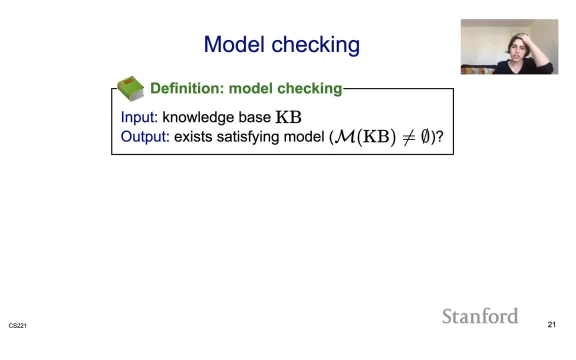 Alright, so going back here, Okay so. so what does model checking do? Model checking takes as an input and knowledge base. And what does it output? It outputs if there exists a satisfying model or not, And if it does, it returns that model. Okay, so it checks if models of KB is not empty. 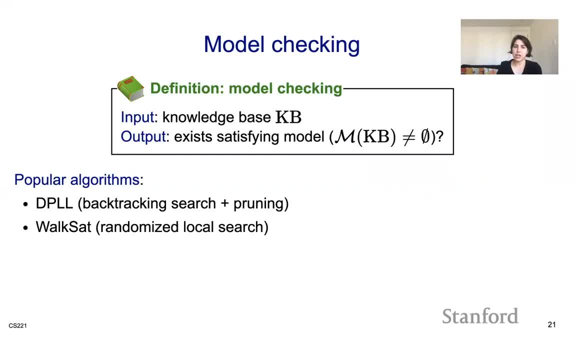 And there are a good number of algorithms out there that try to do model checking, and Some of the older ones is the DPLL is kind of like a well known algorithm that tries to do satisfiability and model checking. What it does is it uses backtracking, search and quite a bit of pruning and quite a bit of heuristic goes into it. 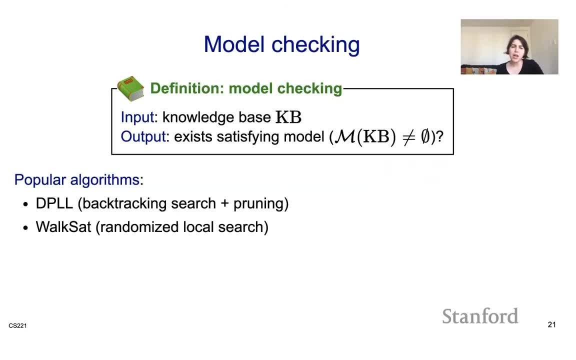 To make sure that it Can solve this problem as fast as possible. Some, some more recent algorithms are things like walk sacks. That is pretty similar to give sampling and it does a randomized local search. There are a good number of Solvers out there. satisfiability solvers out there is. the three is a thing is sad solver that you can look into if you're interested in solving sad problems. 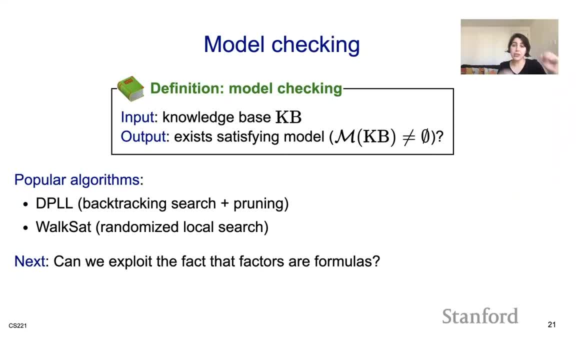 And then, with that, we now have a good idea of syntax, We have a good idea of semantics, and next what we would like to talk about is We would like to Talk about what the formulas get us right, like why do we live in the formula? like, why do we want to even like, look at syntax.